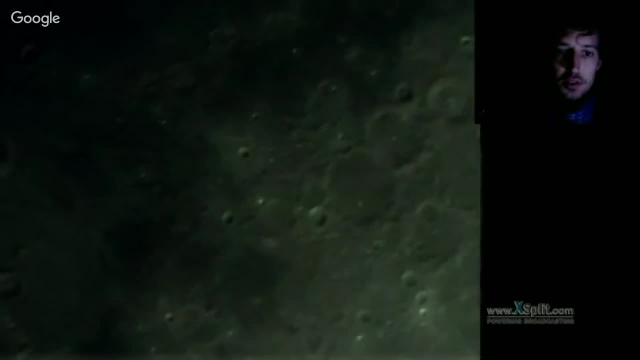 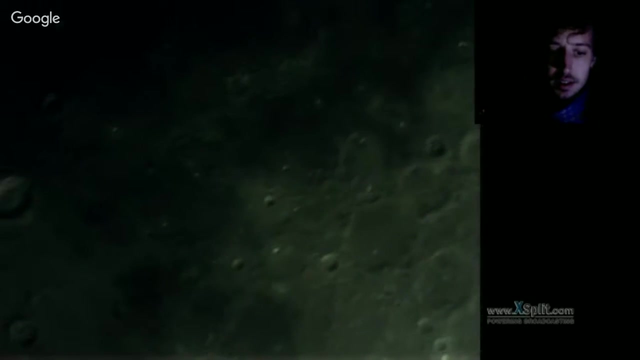 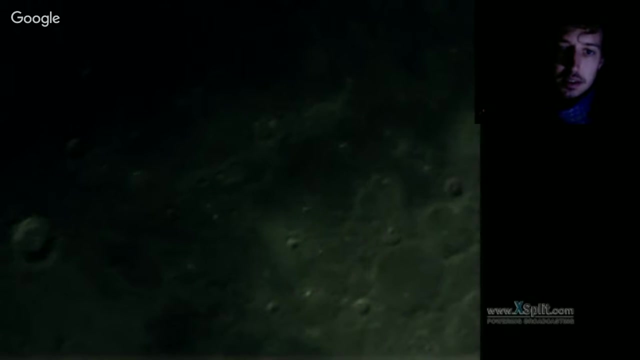 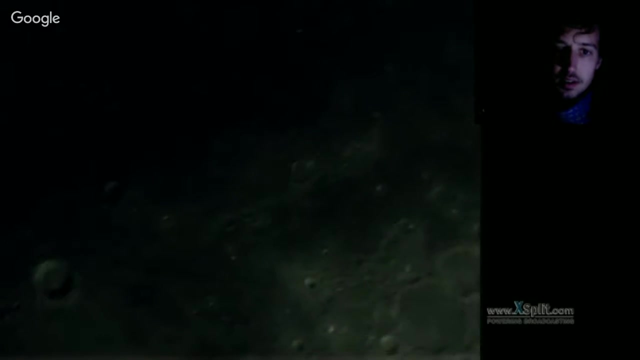 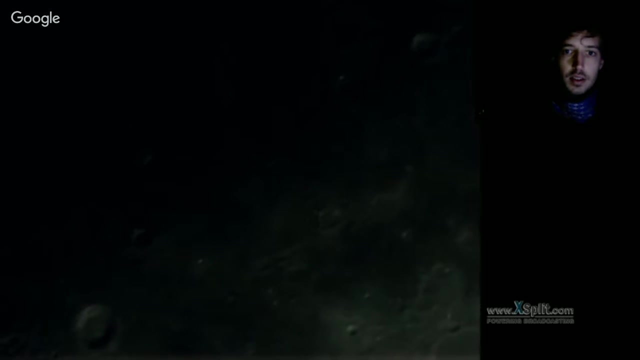 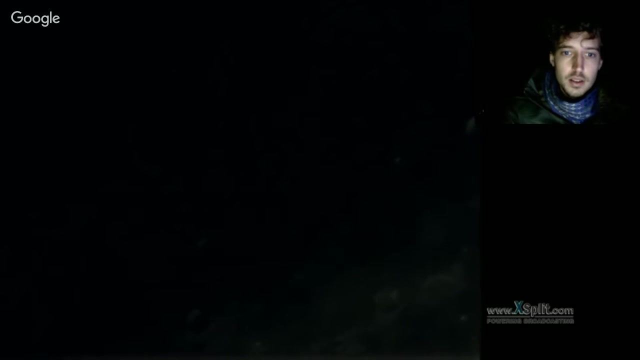 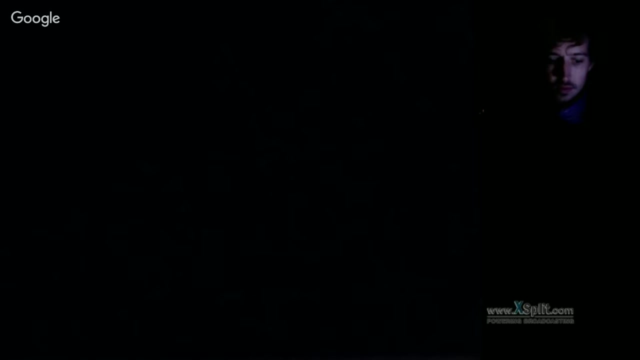 And in a couple of minutes I'm going to introduce what we're going to tell here tonight. Alright, here we go. Alright, here we go. So this eye, this eye here, Thank you, Thank you. So I'm going back to the moon. 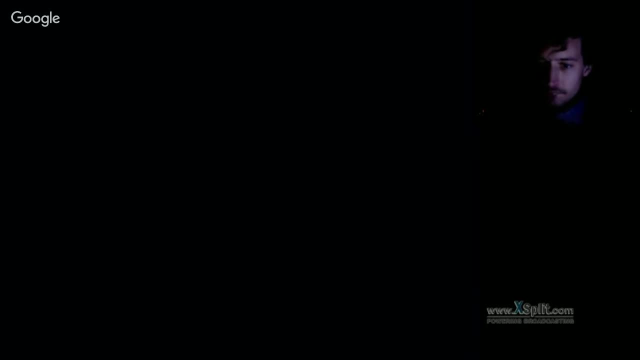 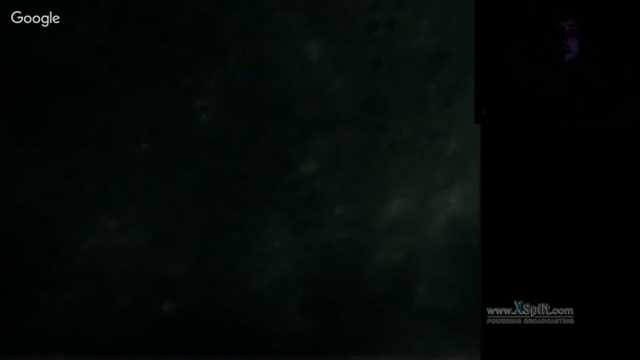 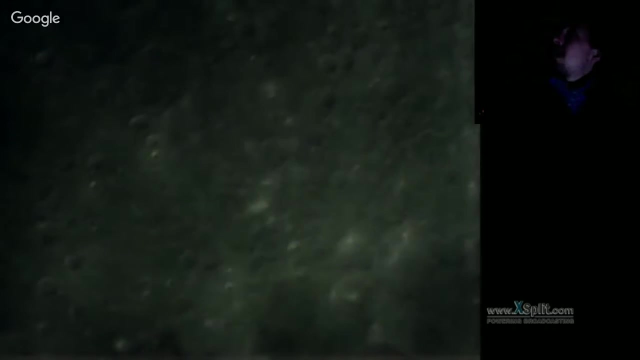 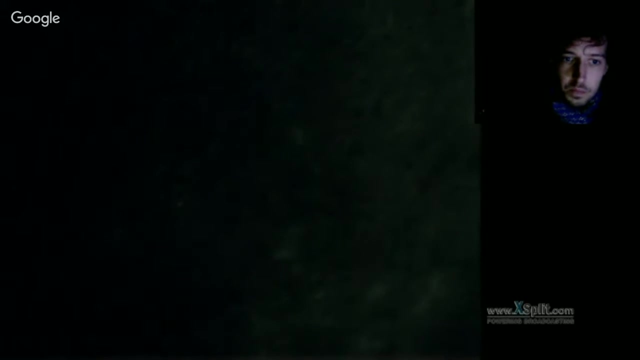 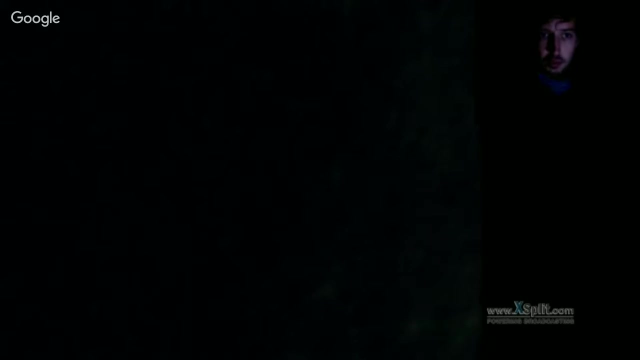 Give me one minute And that's it. Here it is. You see, I have my cloud cover. There's a big cloud coming, unfortunately. Unfortunately, I'm pushing my system. Hopefully I will be able to show you some good stuff. 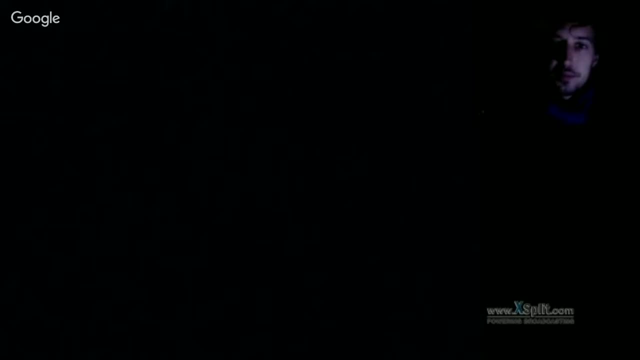 All right, Clouds. You don't like them, So okay, Welcome at this show. This is Astronomy Live show six, And we are planning to tell you a little bit about the basics of spectroscopy, And hopefully our faithful guest, Grant McIntosh, will join us during this show. 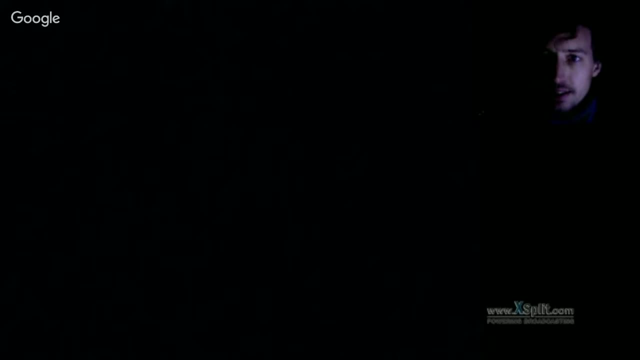 But unfortunately he has some problems with internet due to bad weather. That's possible. So we are very dependent. So we are very dependent on the weather conditions. Sometimes clouds block the sight of beautiful planets and the moon and stuff And sometimes bad weather destroys our equipment. 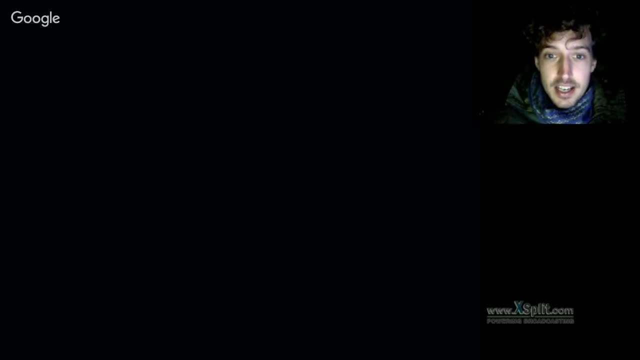 And we cannot help anything about that. So I would like to remind you all that this is our weekly show on Thursdays from 8 o'clock Universal time, So you're very welcome at this show, And each week we will talk about different subjects. 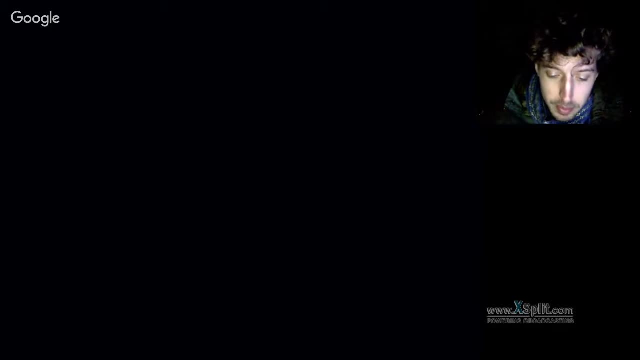 And this week we will talk a little bit about spectroscopy, but also about the Orionids, Because that meteor shower is active at the moment. As you can see, the screen is very dark, And that's true because there is a big cloud in front of the moon right now. 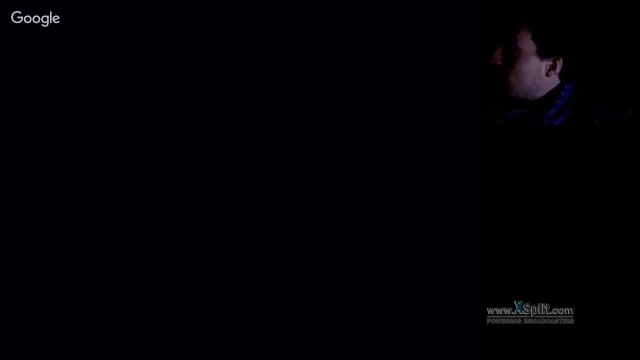 Showing you the moon. There aren't any planets high in the sky, So I'm not able to show you that, And because I'm broadcasting from Amsterdam, which is quite white everywhere, it's difficult for me to show you deep sky objects and stuff. 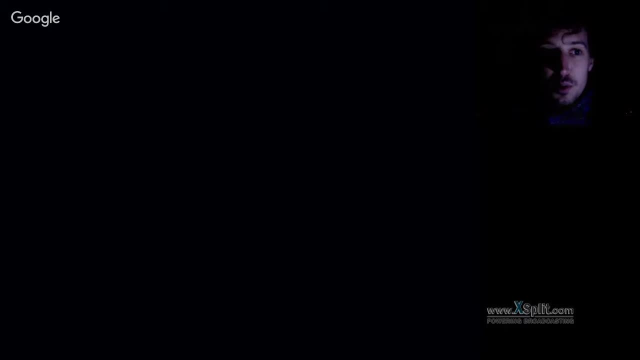 But Astronomy Live should be an international network of telescopes And if you are an astronomer or an amateur astronomer or a professional or amateur, you're welcome to join our network and show the global audience live astronomy as well. So unfortunately I'm not able to show you a lot of deep sky here. 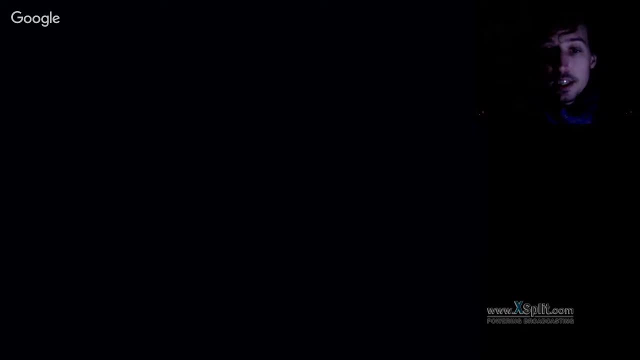 And there's a big cloud in front of the moon right now, But we will talk a little bit about spectroscopy. It's difficult, We're going to go over it. So you're welcome to ask questions on the Q&A. I'm opening the Q&A app right now. 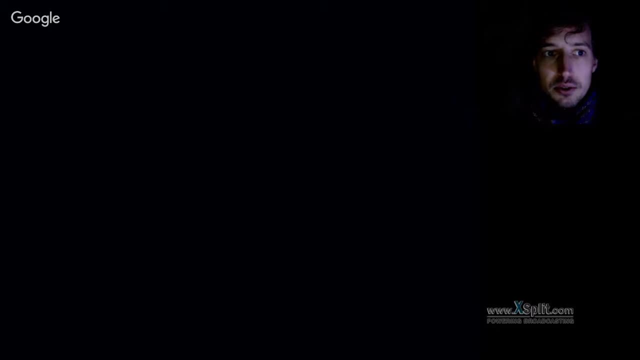 So if you have a Google or Gmail account, you should be able to join our broadcast and ask questions using the Q&A. So I was hoping my dear friend Grant was able to join me, But due to uh damaged equipment, he is not able to uh join me. so, uh, probably we will move the. 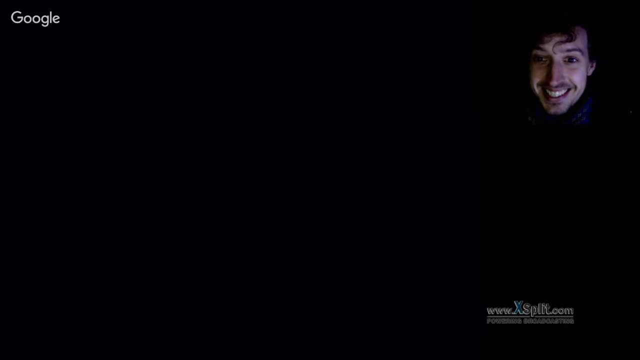 spectroscopy- it's very difficult word for me- uh to next week, um, but the orionids are active and that's very interesting. um. maybe you have heard of the orionids, maybe not, um, but it's a meteor shower that is uh active between the 17th of october and the 25th of 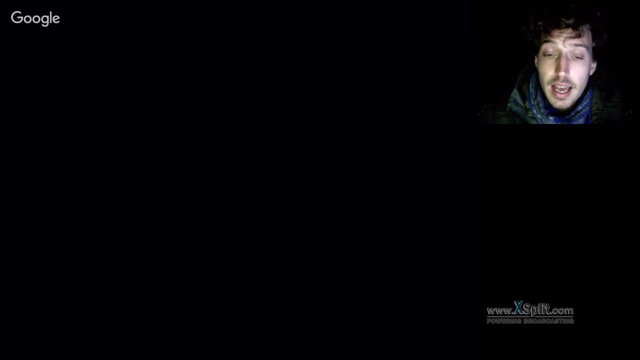 october, currently it's the 22nd, and tonight and yesterday it peaks. so, um, i was hoping, if i am able, to show you some orionids, but i don't have a suitable camera for it, so, uh, i would like to use broadcast as a message to invite others to start streaming as well. um, so the orionids. 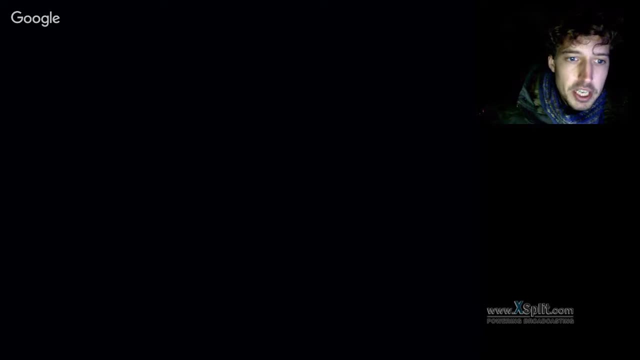 it's a very interesting meteor shower, but not as spectacular, unfortunately, as other meteor showers. during the peak it will be around 30 meteors an hour. um i will show. to start this presentation, i will show you a live map of constellation orion. you see orion in the middle. 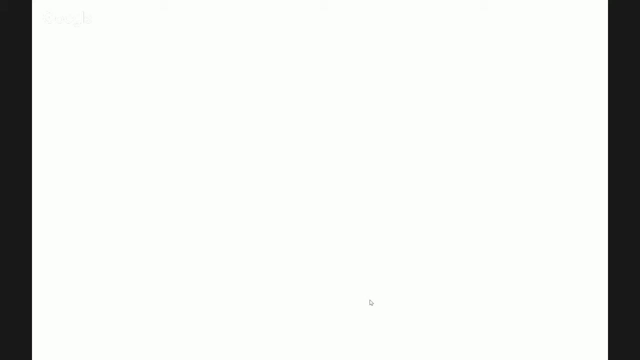 and this is the famous constellation. personally, this is my favorite constellation. so you see here, rigel, that's a knee. this is saip, that's another knee. then you go to the belt, the famous alnitak, alnilam and mintaka, the big red giant beetlejuice. and this one- now, that's not the correct one, but that, this one. 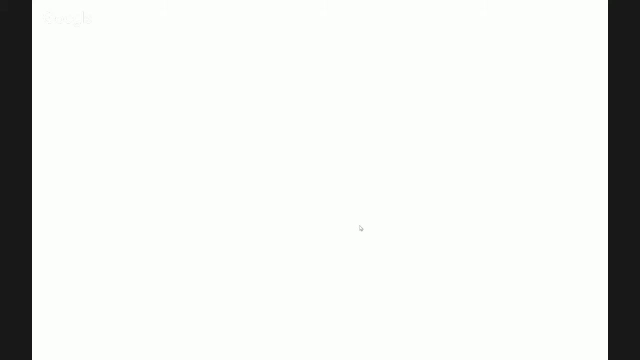 it's a neodymium, one right. talk about the awakushia. mostly there is one on your left and right side of the star. so the belt, two shoulders, a neck, two knees, one arm and one bow, that's the consolation of orion. and when you go to this, 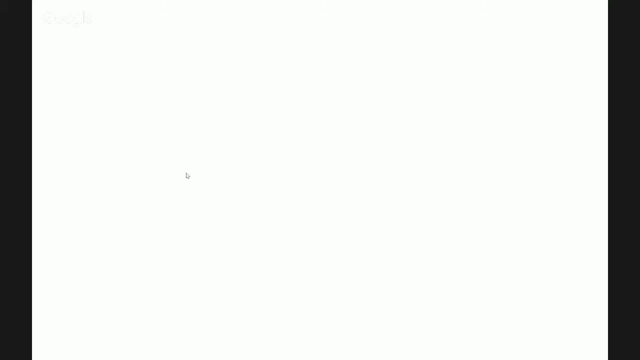 you see this icon. this is the spot, this is the radiant all the meteors are coming from. so it is not wise to look directly at the radiance, because probably you will miss a lot of meteors, but you should be able to look around it because they. 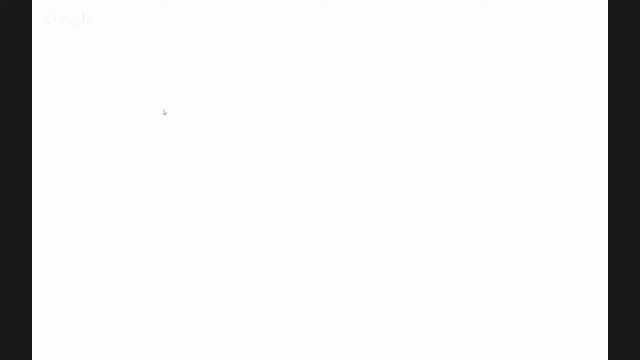 will all radiate from that part, so you will see flashes over here, flashes over here, flashes over here, all coming from one direction. and why is that? to be a dust trail. and that is caused by the dear, no sorry, the comet halley. comet heli circulates the sun every 70, 60 years and leaves. 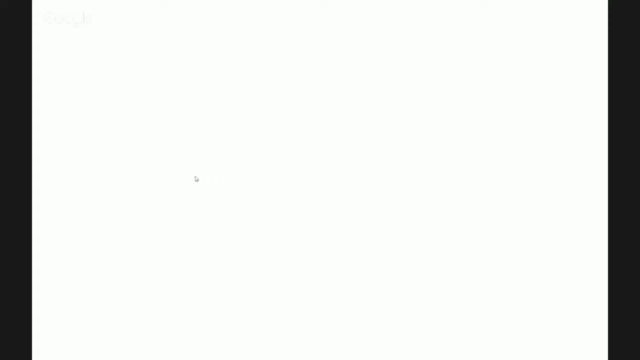 a dust trail, a path of dust and grain, and it's a dirty snowball. so it leaves a lot of dirt behind in space, the dirt that's. it keeps on, you know, floating in space. and when our own beloved earth crosses that dirt path, it, uh, it causes a meteor shower. 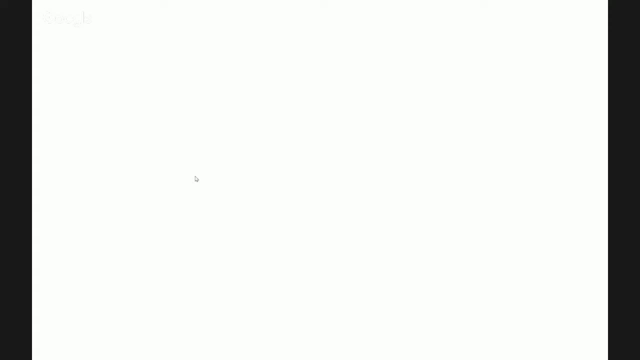 and every time, on the exact location in in space, you see meteors radiating from the same location, from the same spot in the night sky, and meteor showers are called by from what constellation they are radiating- radiating from um. so at the moment it is peaking time, so that means i'm stopping the screen share. 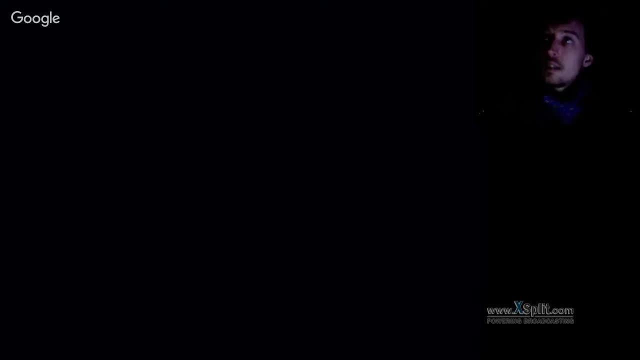 the moon is still not up, so uh, unfortunately. but each year at this moment we are be able to enjoy the meteors from comet heli. comet heli is a well-known comet and, of course, it is named by mr heli. that's normal. you know comets that are um discovered. you know, at this time they are also called to the discoverer. 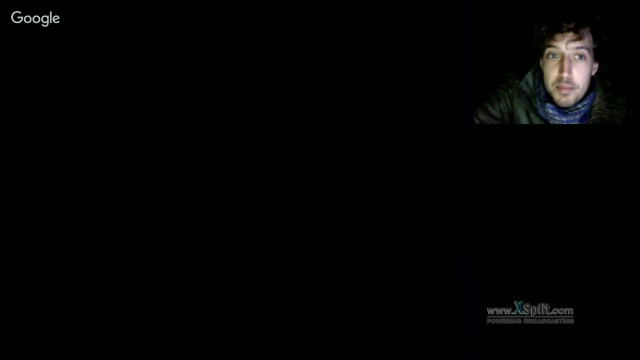 the discoverer is the comet or the meteor shower. the comet bears the name of the discoverer, but uh, mr heli, uh, lived a while ago and uh, well, i think it's interesting to tell about mr heli, because who is mr heli actually? well, uh, 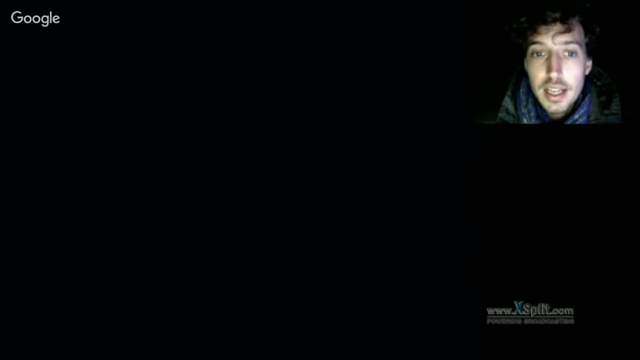 uh, mr heli is called mr edmund heli and he predicted uh that, uh, there was a pattern with comets coming and going, uh by circling the sun, because in history it was already long known that there were a lot of what they called comets, and he predicted that a comet would return in the uh year. 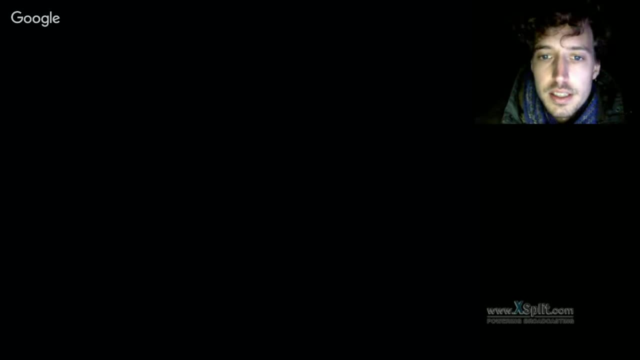 70, 58, and the prediction seemed to be accurate. so and they saw the comet Heli the first time on Hawaii, and it was a kind of interesting phenomena phenomenon and they they thought that it was the presentation of the new upcoming king of Hawaii called Kamehameha one. well so, mr Halley, he predicted the return of the. 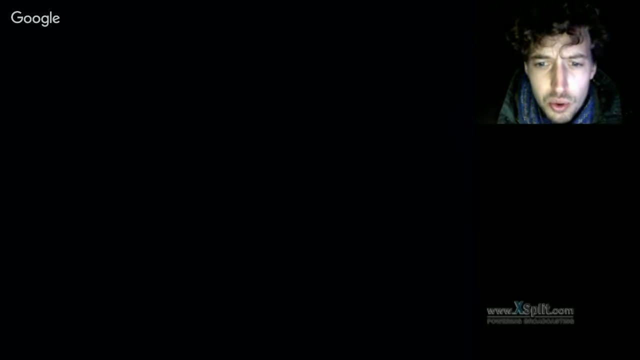 comets and it was already registered in the year 466 before Christ and some people think it was actually the star of Bethlehem. but when they did the calculations was not really correct, knowing that the comet Heli circulates the Sun every 67 years, so the 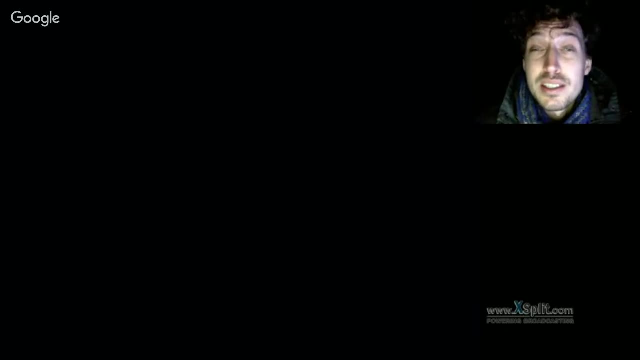 last passage of comet Heli was 1986 already, and it was visible with the naked eye. well, I was one year old at that age, but I remembered a lot of beautiful pictures afterwards, and again we will be able to see comet Heli in the year 2061. come at, Halley is. 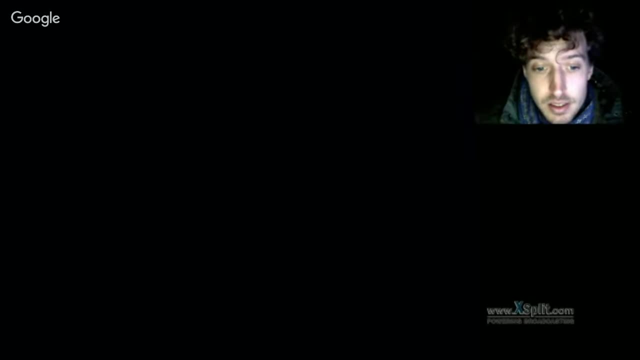 about 16 by 8 kilometers thick, and it has dust and water fountains at around 10 percent of this surface. and then now beto of point for point 0, for which what is our albedo? well, that is, the reflective capability of capacity, capacity of an object, the moon, for. 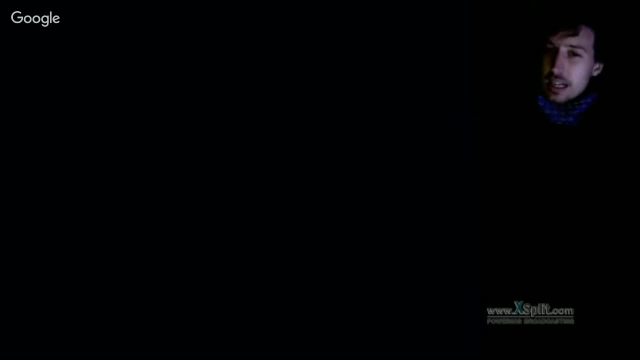 example, has a high albedo, but when there is a cloud in front of it, you cannot. you can't see any thing of it. so that's very unfortunate. um, i think i'm just very unlucky. uh, at the moment, grant's there grant. are you able to join this stream because you have a lovely talk? 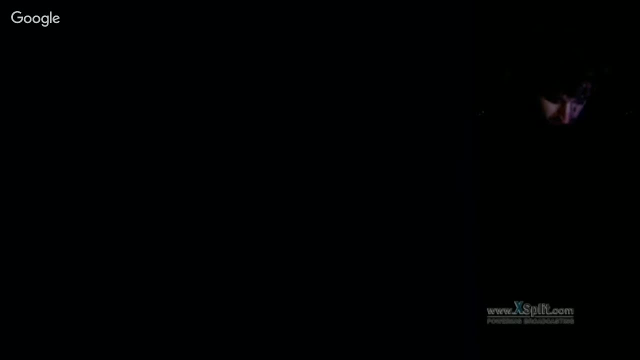 i'm going to send a message to grant because he was planning to tell some interesting stuff about spectroscopy. i'm not an astronomer. i know something about it, but i am sure grant is able to give you a much, much more interesting presentation. um, so please know that we have a q a. 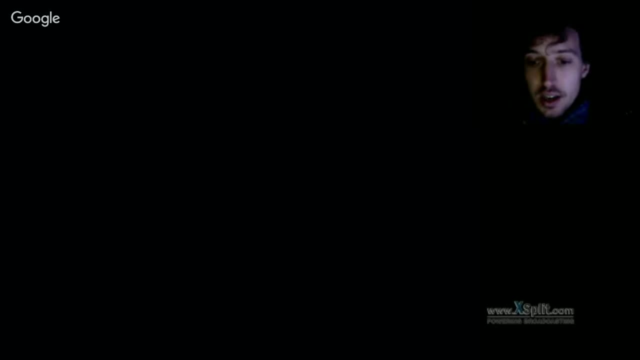 activated at the moment, which means that you can ask a question and i will answer it. you need a google account for it, and then you should be able to find an icon when you hover over the screen. um can ask a question over there and i'm happy to answer it. um, i'm sorry to disappoint you that we. 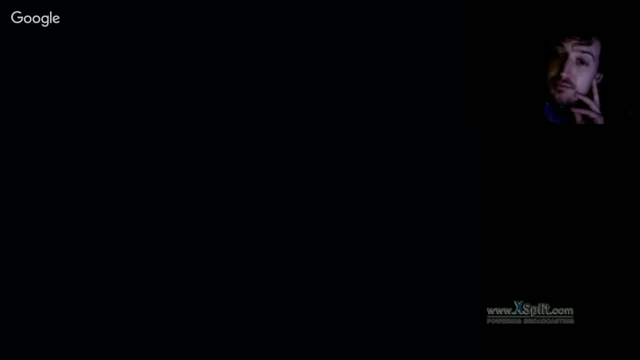 don't have any live stuff um showing for you right now while i'm sitting here in front of my beautiful uh telescope and equipment. but there is a cloud and it does not look good. um, that's strongly, sometimes it's very disappointing and sometimes you're lucky. 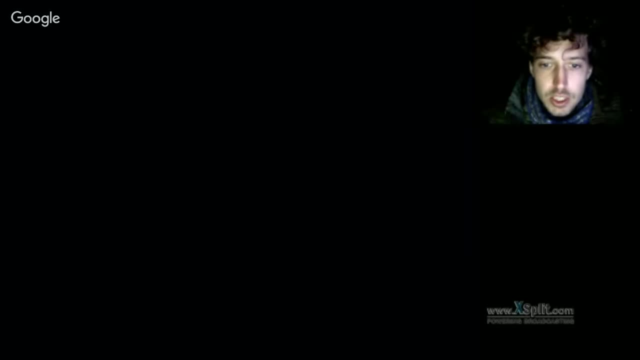 so, um, so that's about the comet heli, um, so the orion is. so i'm showing, i'm, i was trying to show you the moon, but the moon is not very useful during meteor showers, because you don't need light. uh, because the the light from the moon blocks a lot of the faintest meteors that you should be able to pick up. 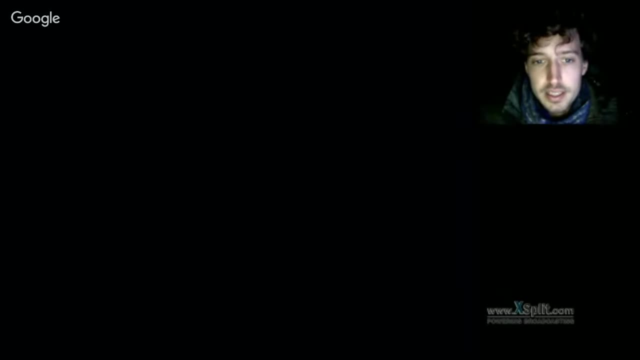 so the moon is currently lit about 71 during peak, and that's today actually, or yesterday, um, and that's uh unfortunate, but sometimes during special meteor showers you have you have no moon blocking and blocking shape between them, but it's always important that the show or spoiling it. so it all depends on the position and the face of 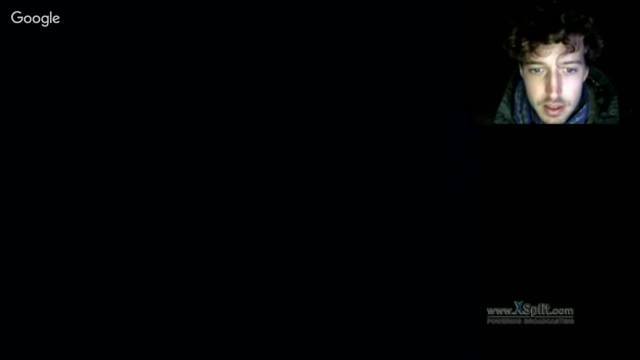 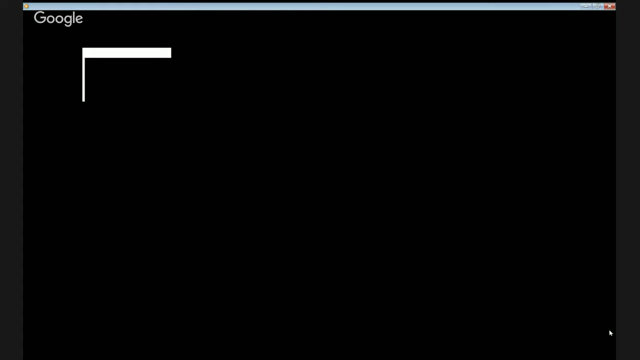 different astronomical objects for you to be able to enjoy a show, I can show you a nice movie of a recorded meteor shower and let me get that for you. okay, one second. this is a nice movie of mr James mg, if I'm correct, and you see. 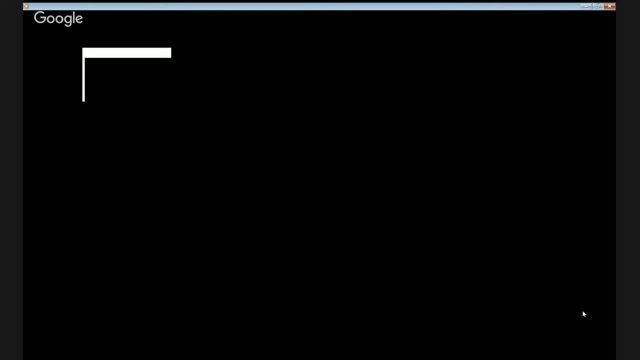 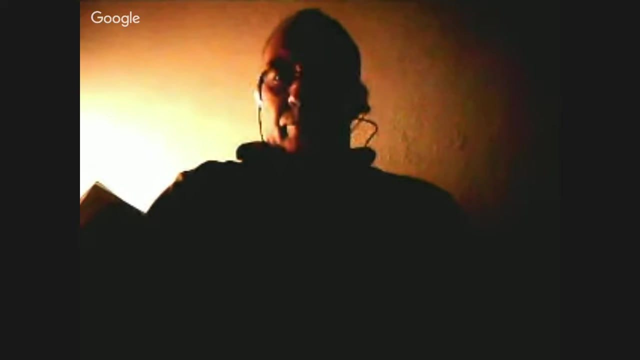 some airplanes passing by. you see the constellation of Orion Here, an actual ball of hers is the radiant. sometimes you see Nietzsche's, and here you see beautiful planets: Venus with Jupiter and Mars, yes, in the video, but I see a beautiful man from Great Britain: hello Grant, hello Xander. apologies for tonight. we'll talk later. okay, no problem, man. 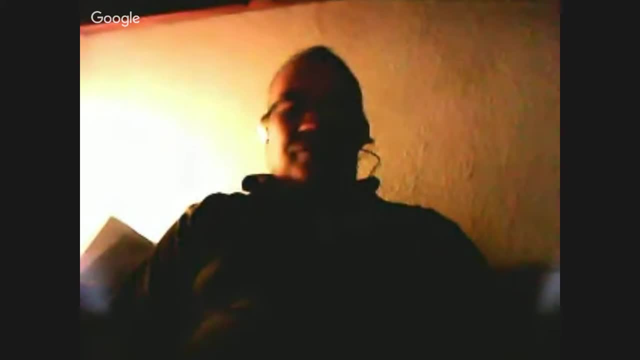 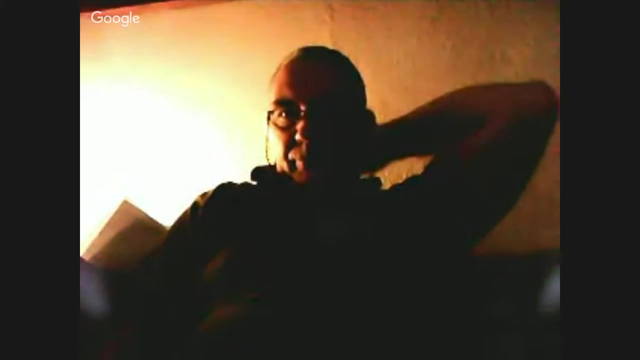 so what we're looking at tonight? yeah well, um, I'm looking at a night sky which is currently about 60 and covered with clouds. uh, earlier on it was uh looking good, but now I see some holes in the sky. hopefully I will be able to show you a couple of minutes of the moon, but it doesn't. 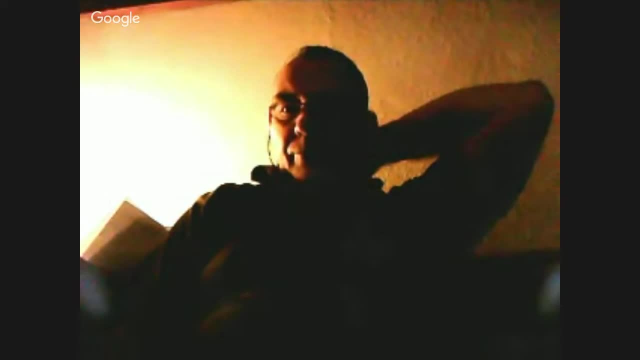 look good. unfortunately, uh, you're still still experiencing problems, unfortunately, with, uh, the internet. yeah, I'm gonna make a couple of phone calls tomorrow because they assured me it was repaired, Xander, and it's not. I mean, I just couldn't stay on for any length of time. 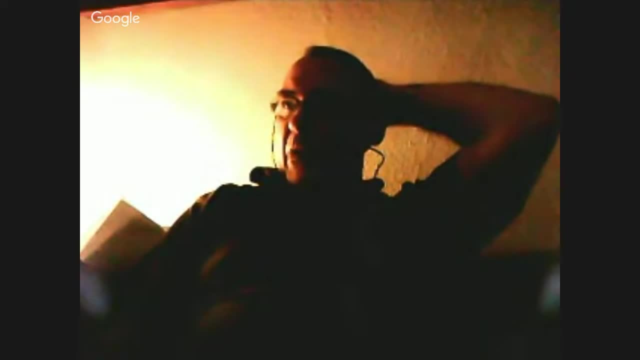 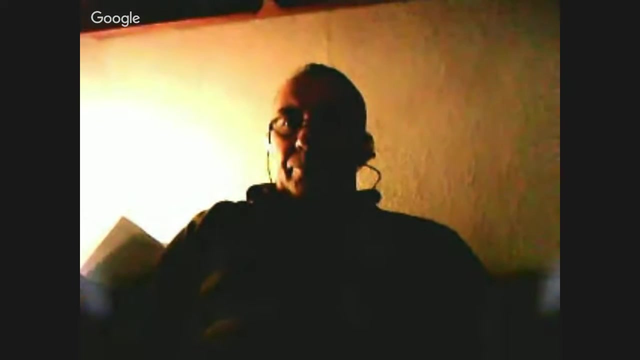 this evening. so, uh, I've brought the, I brought the equipment home with me, so, while um, I'm on my, I'm back at home now. so, um, I'll, uh, I'll get that sorted once and for all tomorrow. yeah well, uh, no problem, no apologies needed. it's uh, that's uh astronomy as well, sometimes. 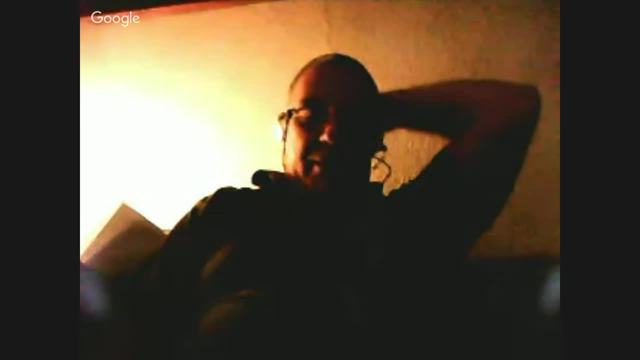 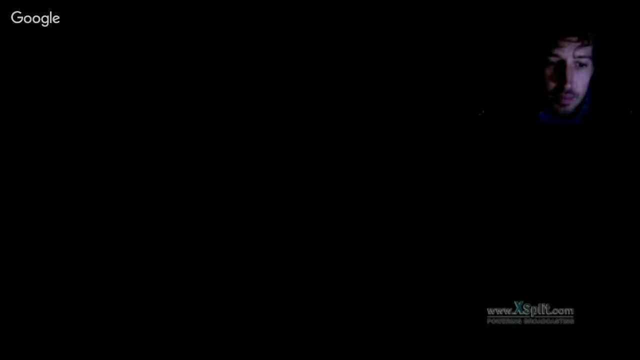 you're lucky and sometimes you're not. yeah, um, but as I said, it clouded as well. I had the moon earlier on. it was lovely, um, really nice. view of Plato in the Alpine Valley, yeah, and then the clouds came. typical, yes, very typical. well, uh, I found some nice uh movies of, uh, the meteor shower. um, on. 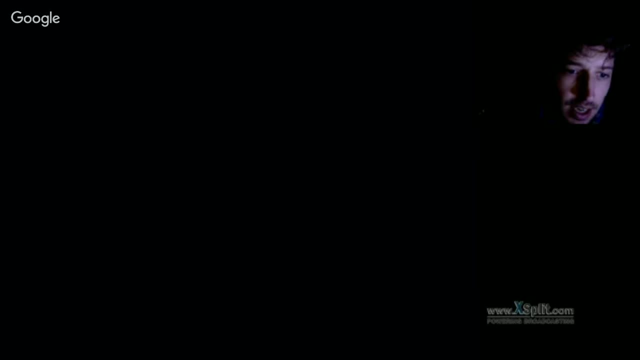 um on the internet and, uh, I was with, I was uh, I would like to share. uh, let me check one second. I found uh an interesting video from oh boy leaving the style from Eastern county, and I'm um, okay, I will show you the video as well. um. 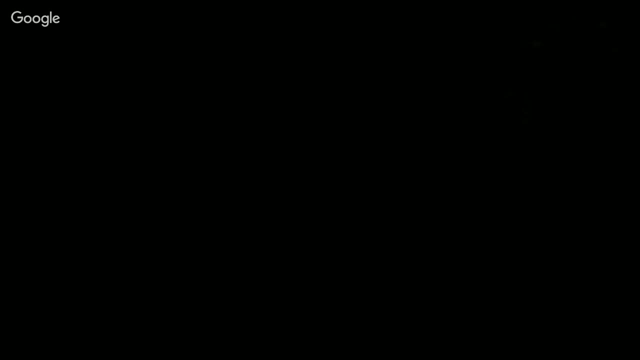 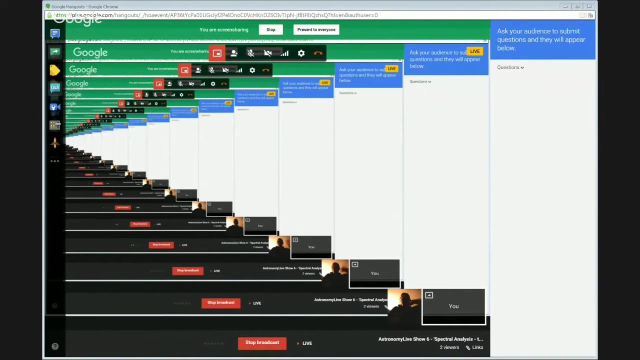 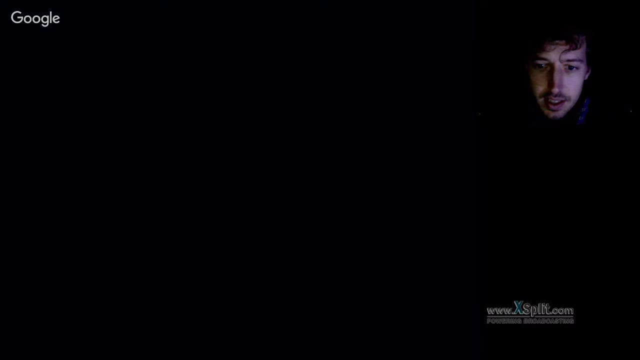 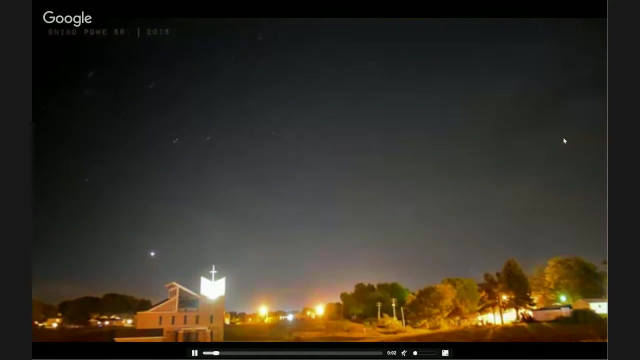 let me uh, that's not good. um, do you see a video? no, I just see quite a lot of uh screen. yeah, okay, that's not good, let me retry. so this is a video. it's a time lapse. yep, probably some. you see play 80s M45. yeah, I can see that. 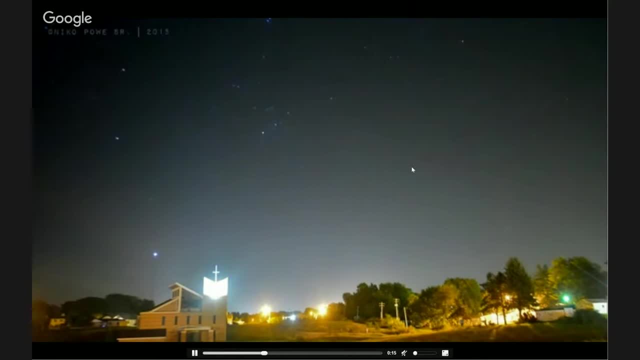 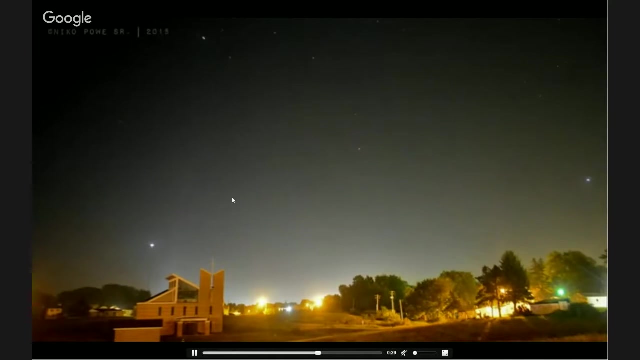 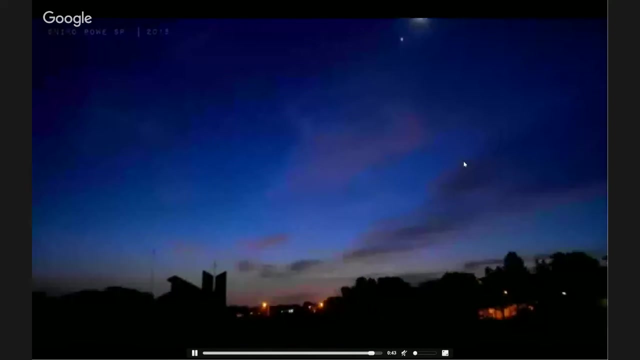 Taurus. a few satellites going across as well, yeah, but also some, uh, V2. right, and I love the end of this movie. you see Planet Venus conjunction, Planet Venus- this is Geminids- and Planet Venus and Jupiter and Mars. wow, that's penis, Jupiter and Mars- a little bit below it, yep, I can see that. that's fantastic, wow. 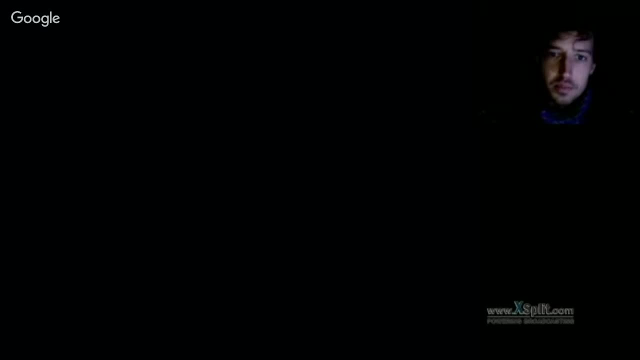 beautiful. yeah, I love that one. it's really cool, um, really cool time left. so, uh, thanks for that. uh, well, I just found the video. are you looking at Stellarium at the moment? no, you're just a blank screen at the moment. no, um, but it's. you can manage the sound effect. just do it barehands. oh, goodoooo, bro. J tylerium does Th Mesテera Pediatricsаче Touaregion Radiation Show, microgravity Helper, Dng Glottium cleaner, Time Lapse & Radisson Poly grande schluck and seminar onこう. 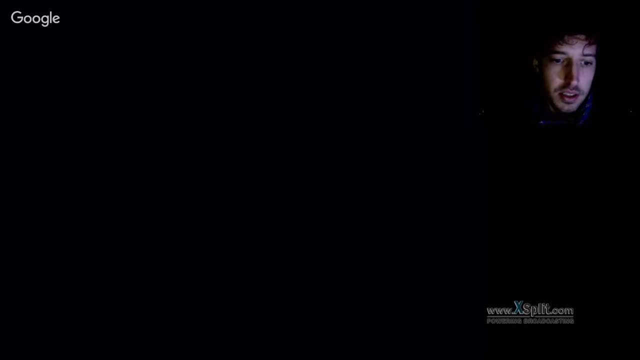 you're just a blank screen at the moment. you're talking to me. yeah, yeah, i'm talking to you. yeah, yeah, i'm actually back home now, xander. we just left the observatory. there was no point staying up there because of the the cloud. yeah, yeah, and obviously no internet connection. i wanted to try. 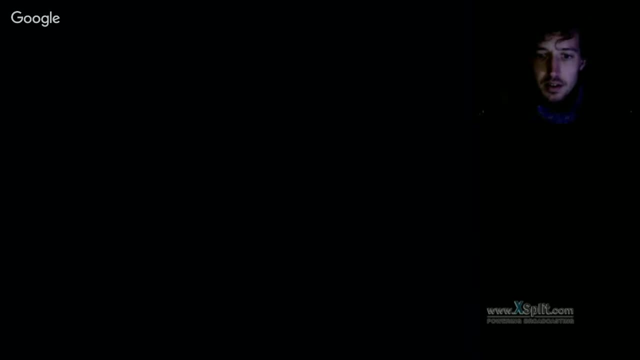 and get back home so that i could actually speak to you on my main internet here to let you know what happened. yeah, yeah, well, um, uh, that's no problem. people have to know that we're, you know, trying our best and uh, sometimes they get a nice show and sometimes they don't. yeah, um, but. 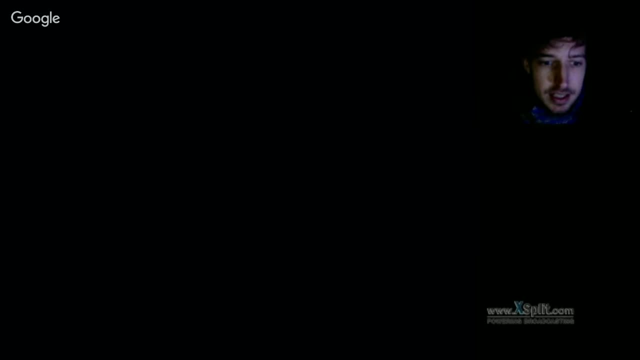 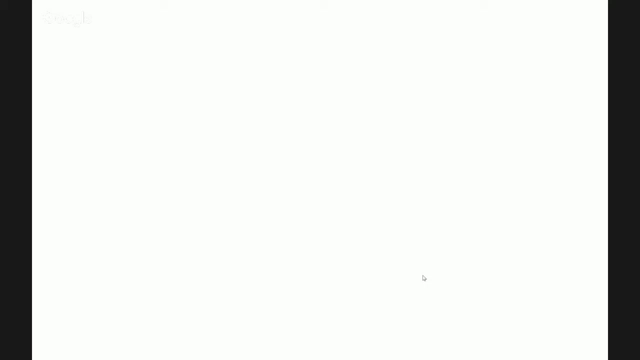 uh, that's no problem, that's uh, that's how it works. um, maybe we could. um, i'm showing stellarium at the moment. do you see stellarium? i just see a white screen at the moment, xander. oh, that's still a white screen. yeah, still a white screen. okay, well, that's, that doesn't work, then i don't. 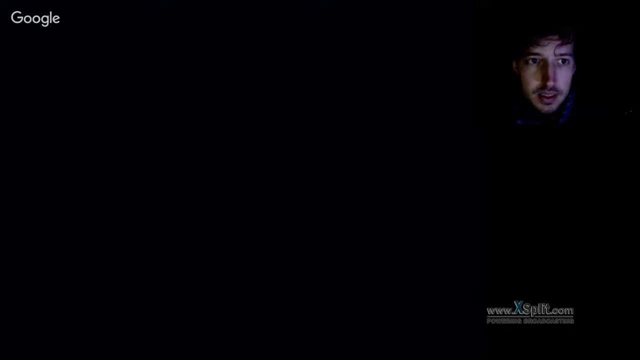 know why, but, um, that's not how it should be. and now you see, you see me, i can see you in the top right hand corner. yeah, yeah, okay. so, um, what is your favorite i? i absolutely love m14, 2 and m43- the orion nebula. yeah, a lot of people just think it's one messy object, but it's actually. 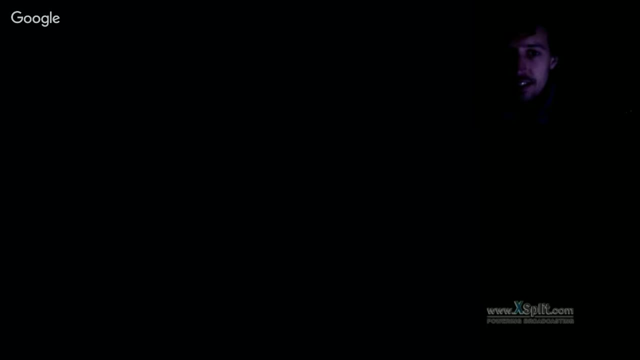 two um and that. that is it for beginners to well, to to find with a telescope and actually image even with a dslr camera, that's one of my favorite objects. yeah, and orion, that was the first object i turned uh into, uh, when i was using my uh first dslr camera. 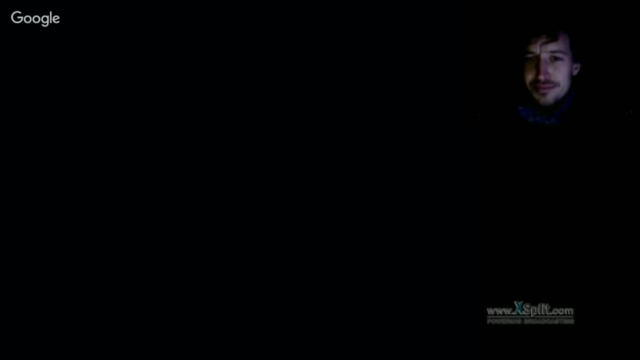 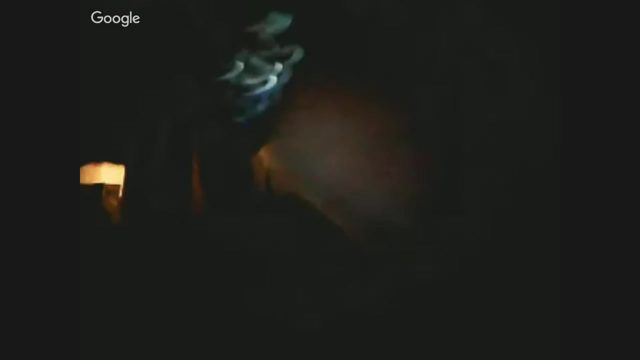 well, um, but i i was much better in webcam astrophotography of the planets so, uh, never got used to that. yeah, yeah, i'm just plugging my laptop into the mains so the body doesn't go flat. just need two seconds. oh damn, big cloud there's. there's not much of a wind, so it goes very. 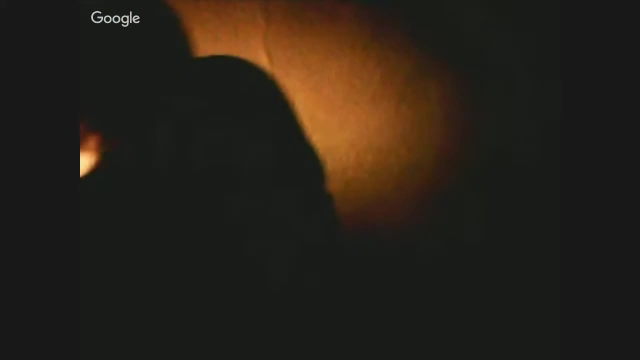 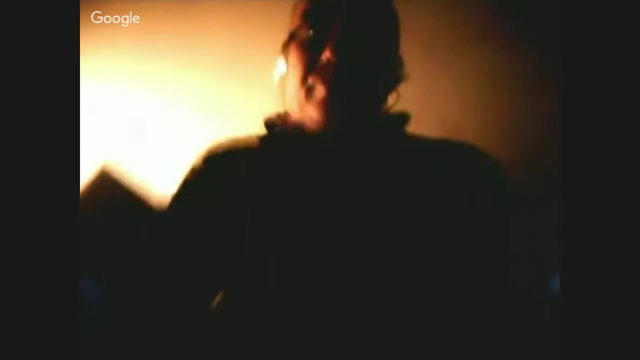 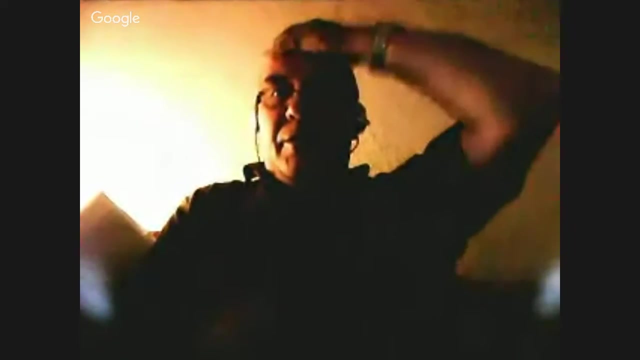 very slowly, some holes, you know, i don't know, uh, how about cornwall? but uh, in the netherlands, when it is, when it is uh clouded, especially in amsterdam, totally, totally clouded, which, and then you know you don't have to wear lights on your bicycle, for example. yeah, yeah, it's orange, the whole sky is. 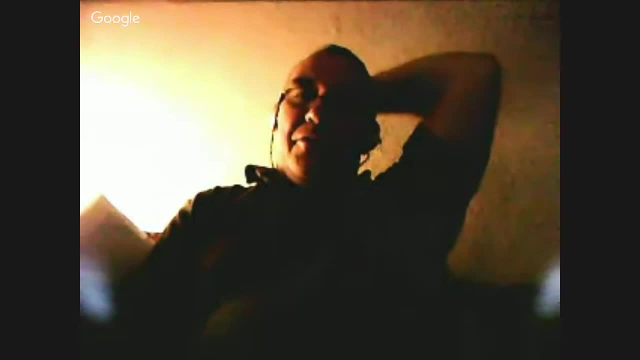 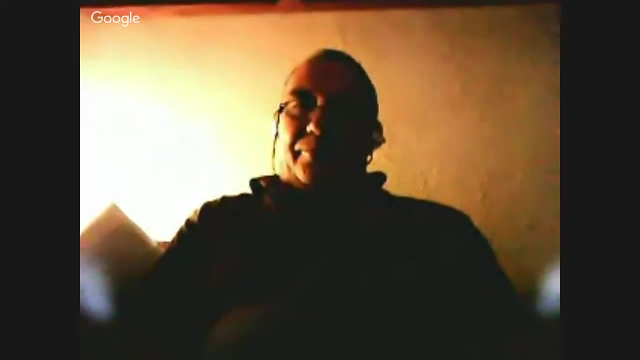 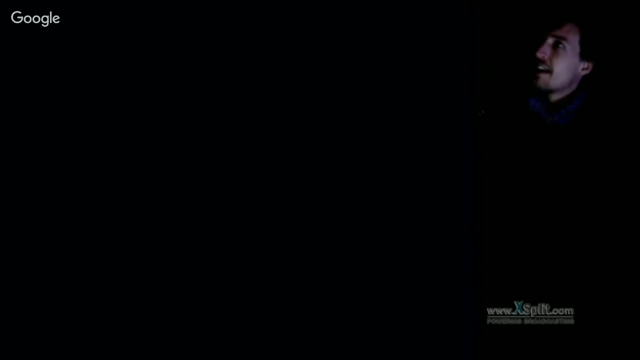 orange. uh, you listen to your radio interview as well, xander, very impressive. thanks, man, it was really cool to do. it was on the national um, on the national radio, uh, as i messaged you, and uh, uh it was. we have, like, uh, our, our, uh eight o'clock news. yeah, yeah, it's uh called. 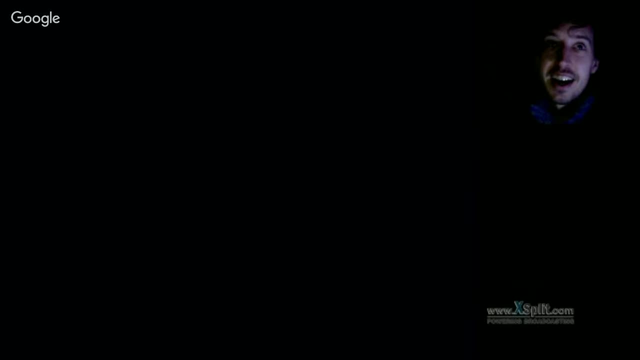 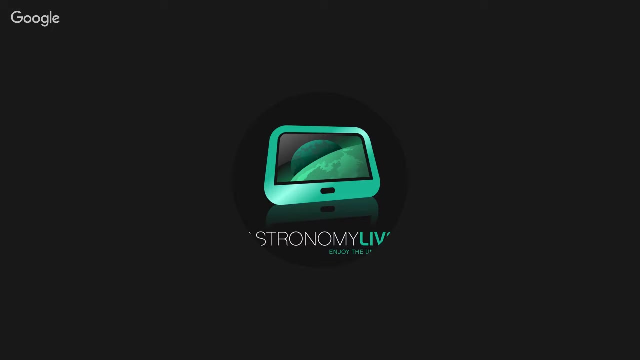 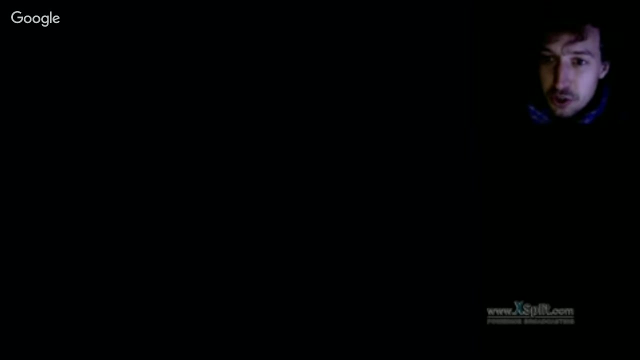 nos and I think six months ago there was a guy with a gun who entered the building of our national news station and uh broke into the studio with a gun and uh forced uh the person present, the guy presenting the news with a gun, to um let him uh be on the eight o'clock news and 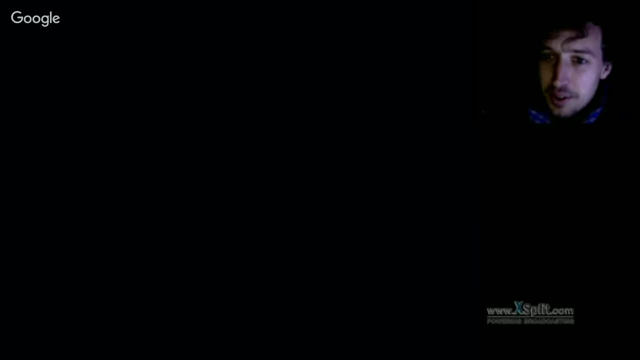 it was like: uh, what did you talk about the, the air force? uh, when you go to the security and uh, yeah, i don't know what that is, and i was just then. uh, i got uh in the retrouve. oh, a dashingracer. before that i took the. 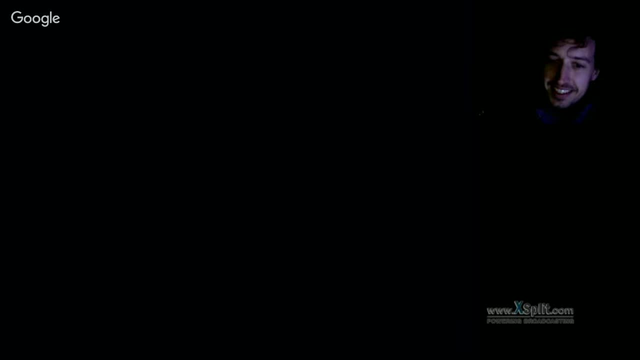 yeah, carrying a telescope with me and it wasn't loaded. it wasn't loaded. no, yeah, maybe. yeah, we need to get one minute, I think less, but I think the moon will pop up. yeah, well, the room is looking fabulous here. earlier on I had my telescope on it with a, with a camera, and I thought, yeah, we're gonna get. 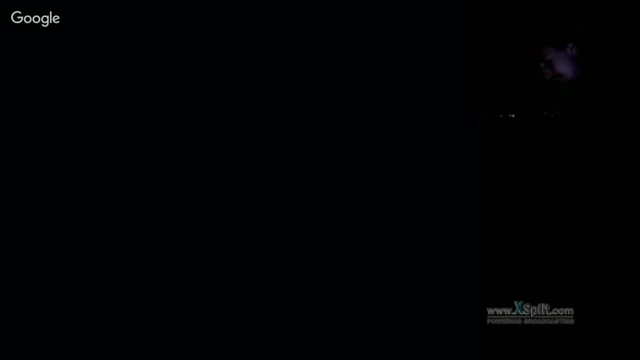 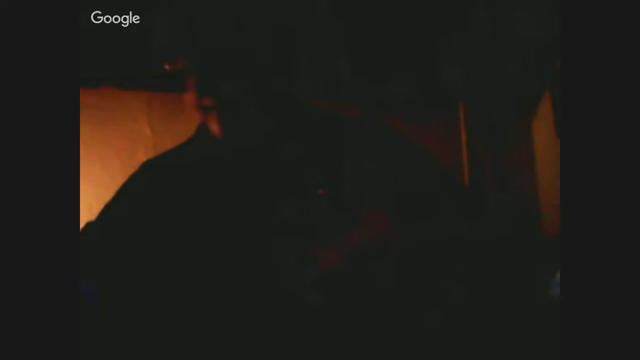 something to broadcast later on? yeah, so we didn't see anything. yeah, problem with your enhancer? yeah, it's an amplifier that we use. if I don't use the amplifiers under, yeah, we don't get a good signal. yeah, so I think that was a problem. but I will have a look tomorrow and get that sorted and I think the 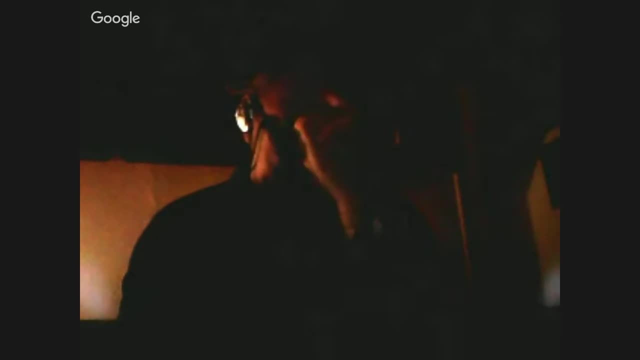 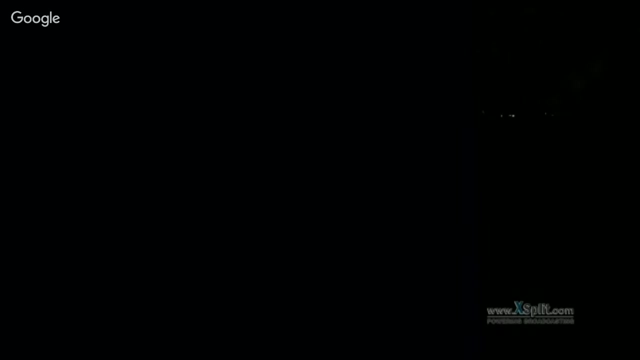 weather is going to be quite good for tomorrow night. I'm going to check again tomorrow, so probably do a broadcast tomorrow as- and I'm just check- everything's working okay. then we can get- we get that spell well, that spectroscopy lecture already, and it's just the case again- a decent 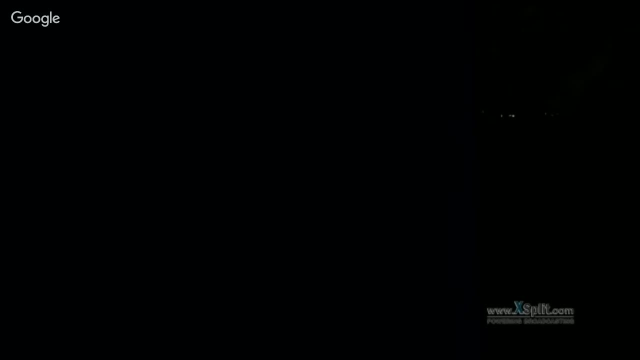 night, because what I want to try and do is put one of the spectrometer gratings on to Vega and broadcast the star and its spectrum. okay, yeah, so for everybody who is watching this broadcast live or if you are watching it afterwards, we are looking for more broadcasts to go in a show on a 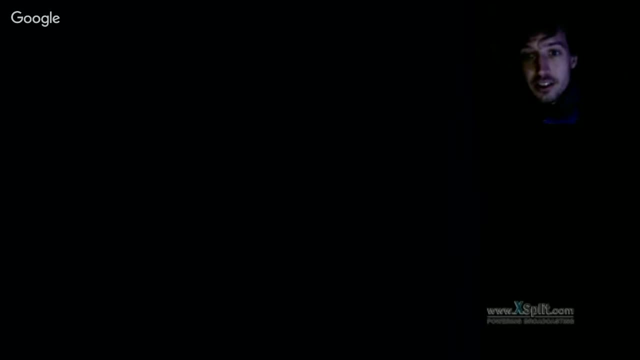 weekly basis. feel free to contact us on astronomy light com. that is our platform, and it's a platform to do this, and that's our platform. we'll see you in the next video for amateur and professional astronomers to join us and I will show you the moon. 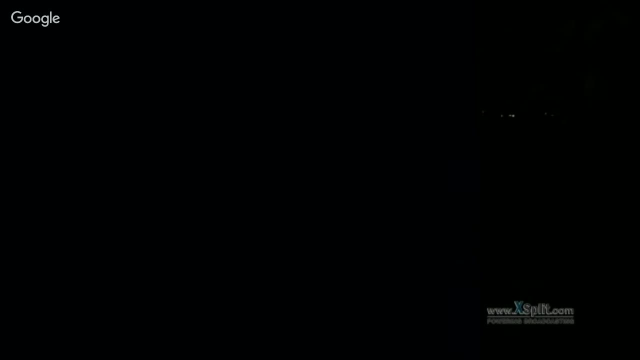 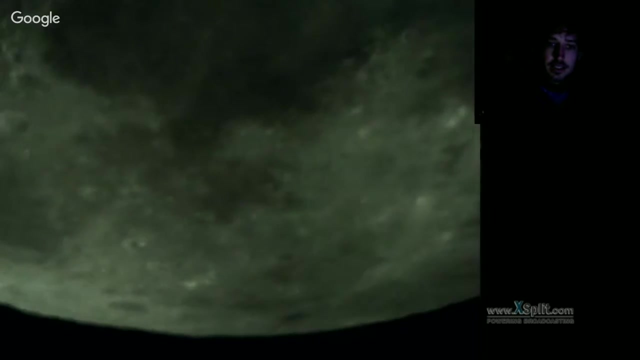 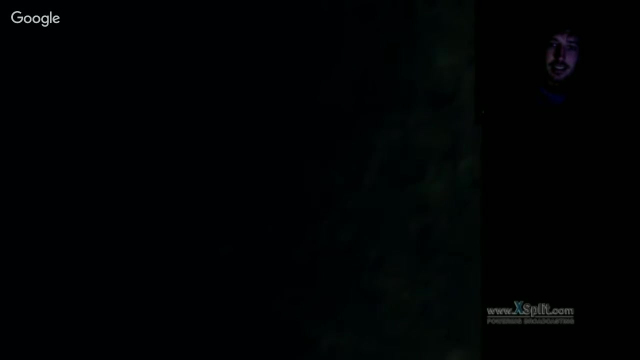 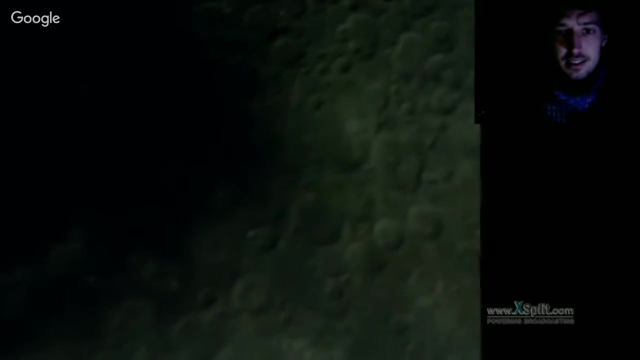 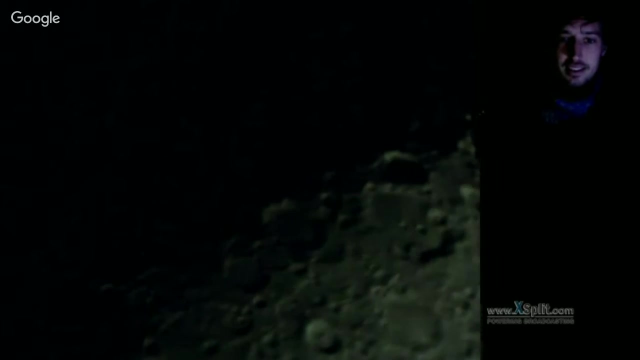 and I will put my telescope on now. still too much clouds. we have to be patient. our doesn't look good. yeah, you saw something and one second. yeah, yes, that's a great cameras under. oh yeah, this is a nice part. look at this. this is a nice part. look at this. 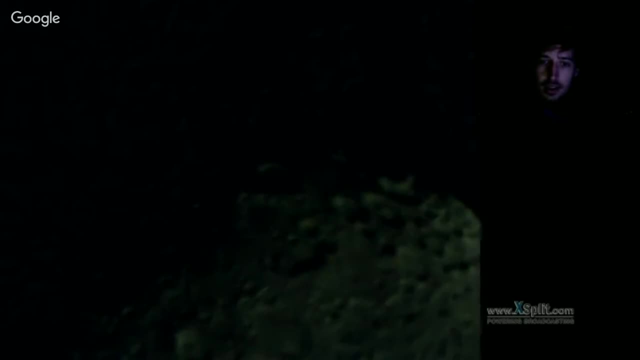 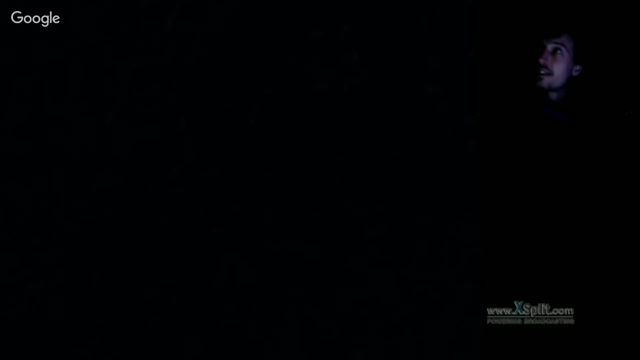 looks like, yeah, yeah, that's clove. looks like, yeah, yeah, that's clove. yes, yeah, yes, enjoy it very quickly, got 80% covered. yes, enjoy it very quickly, got 80% covered. yes, enjoy it very quickly, got 80% covered here. oh, in the beginning of the 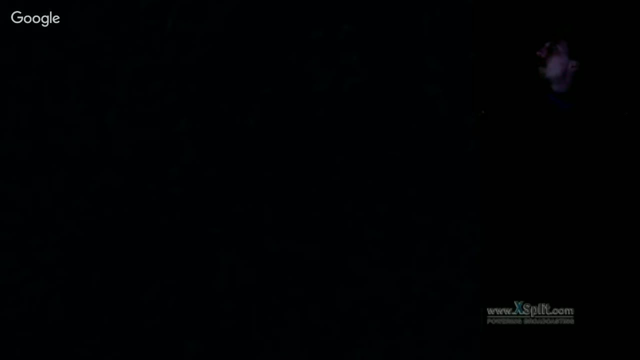 here, oh, in the beginning of the here, oh, in the beginning of the evening, it looked very good evening. it looked very good evening. it looked very good. but now it's done. so i already talked a, but now it's done. so i already talked a, but now it's done. so i already talked a little bit about the. 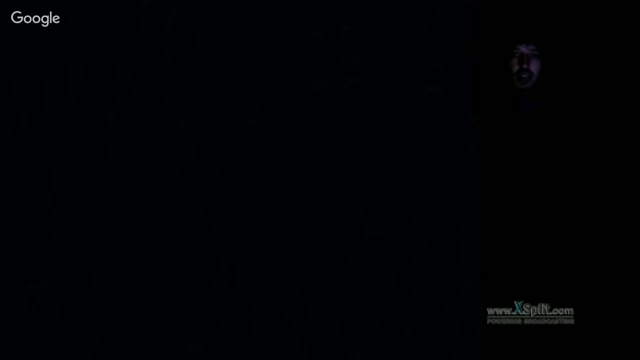 little bit about the little bit about the rhinitis meeting tower. so it peaked rhinitis meeting tower. so it peaked rhinitis meeting tower. so it peaked yesterday night, yesterday night, yesterday night. yeah, we saw a couple tonight. well, ken saw. yeah, we saw a couple tonight. well, ken saw. 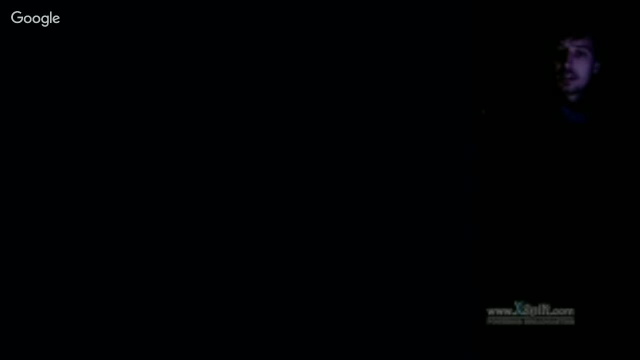 yeah, we saw a couple tonight. well, ken saw a couple, a couple, a couple. uh, i saw one um and then it clouded. uh, i saw one um and then it clouded. uh, i saw one um and then it clouded. oh wait, oh wait, oh wait. 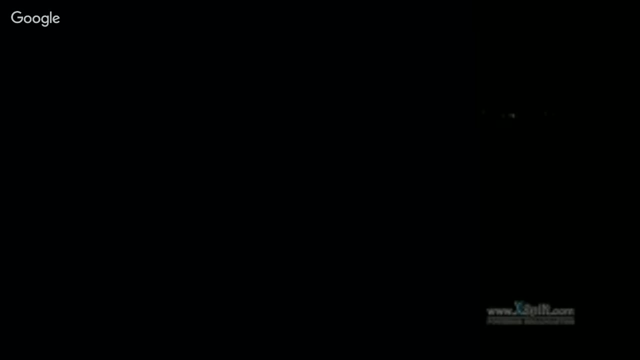 come on, i saw kim saw a couple. i saw one, and then i saw kim saw a couple. i saw one, and then i saw kim saw a couple. i saw one and then it clouded. i was getting exactly the. it clouded. i was getting exactly the. 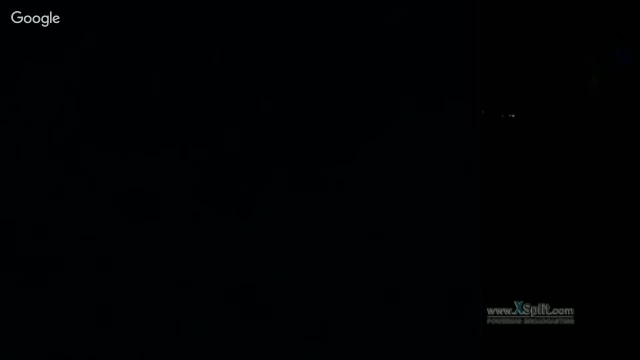 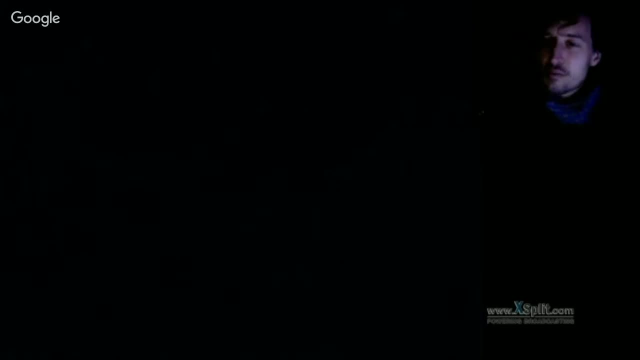 for all you guys entering during this show, welcome at astronomy during this show. welcome at astronomy during this show. welcome at astronomy life, life life. actually probably not or not. um, actually probably not or not. um, actually probably not or not. um, we are like broadcasting. we are like broadcasting. 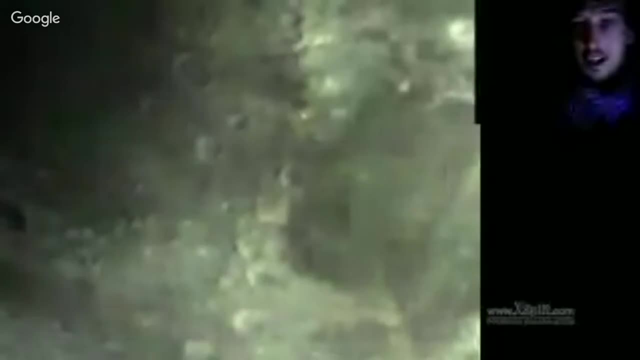 we are like broadcasting thursday and try to get you something thursday. and try to get you something thursday and try to get you something to show you something like you see right to show you something like you see right to show you something like you see right now. 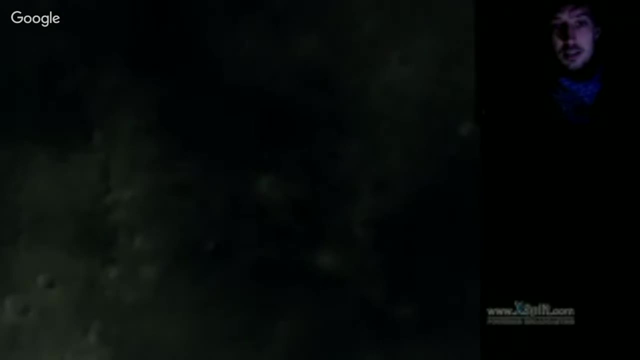 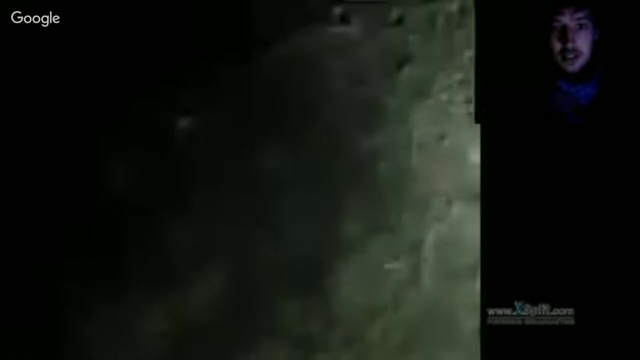 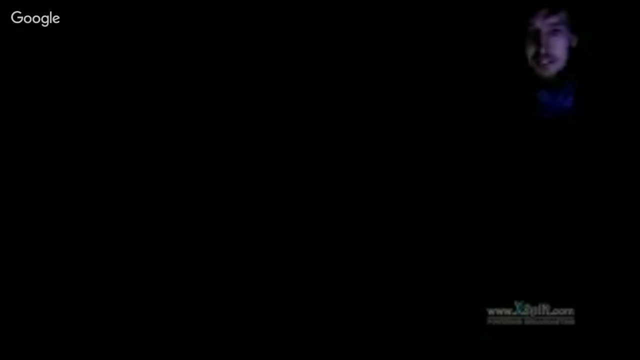 and that's our moon, and that's our moon, and that's our moon. ah, that's beautiful. yeah, that's clavius. yeah, it's fabulous. i like the moon when- yeah, it's fabulous. i like the moon when- yeah, it's fabulous. i like the moon when it's a space zander, because you can see. 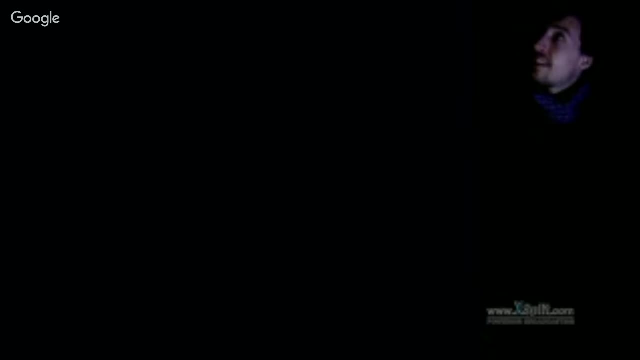 it's a space zander because you can see. it's a space zander because you can see all the shadows, all the shadows, all the shadows, and the ends of the craters for the and the ends of the craters for the and the ends of the craters for the causing the sun causes. yeah, 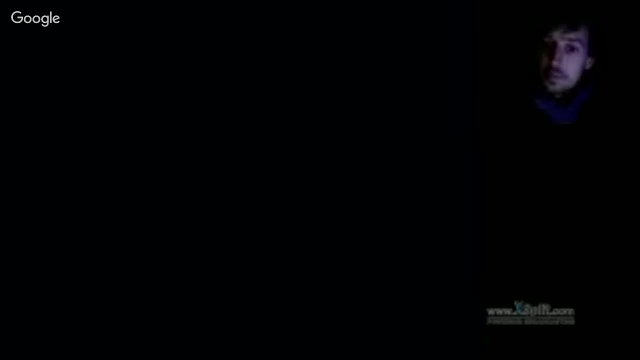 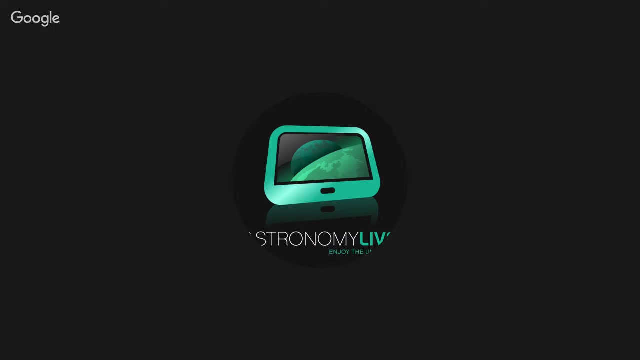 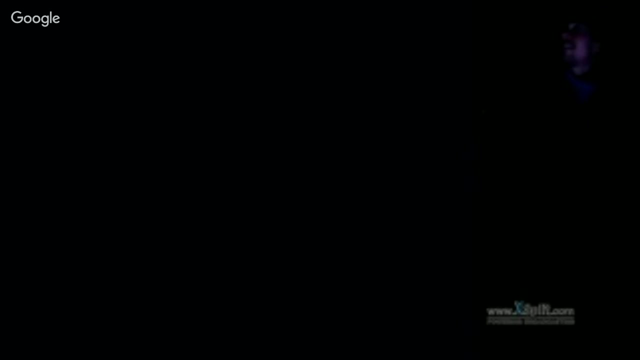 causing the sun causes. yeah, causing the sun causes. yeah, yeah, you too, yeah, you too, yeah, you too. you see some lights in the back. there's a carnival over here. yeah, yeah, this is this is a ferris wheel. yeah, this is, this is a ferris wheel. 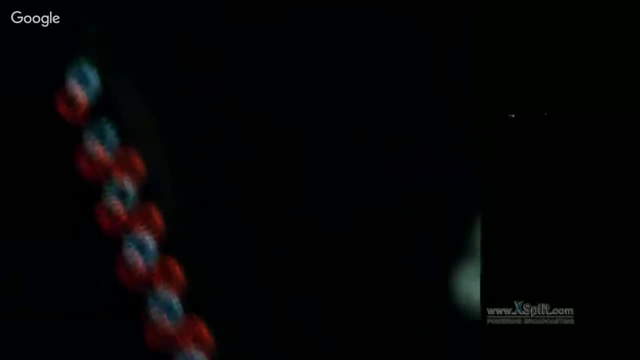 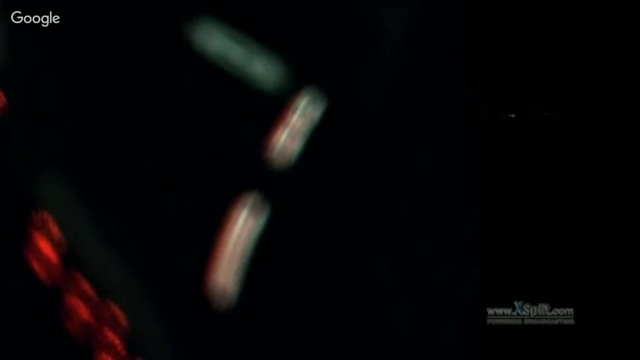 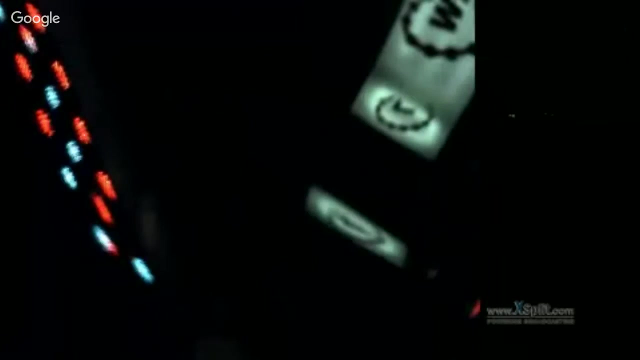 yeah, this is, this is a ferris wheel. you should have said it was the dumbbell. you should have said it was the dumbbell. you should have said it was the dumbbell nebula, that would have worked. at least that's not clouding out, zander. 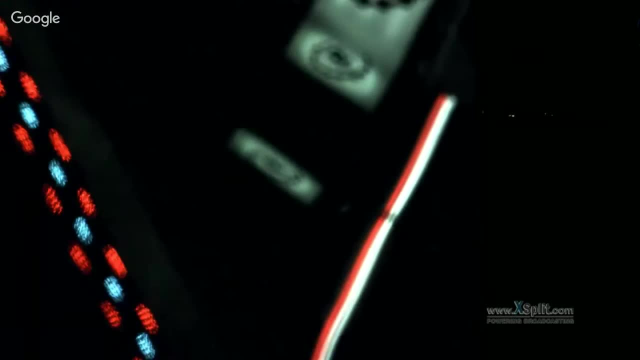 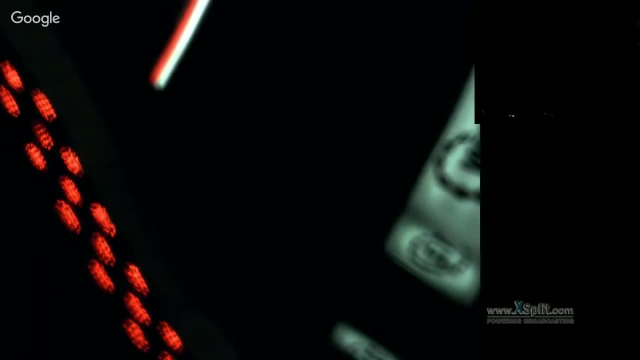 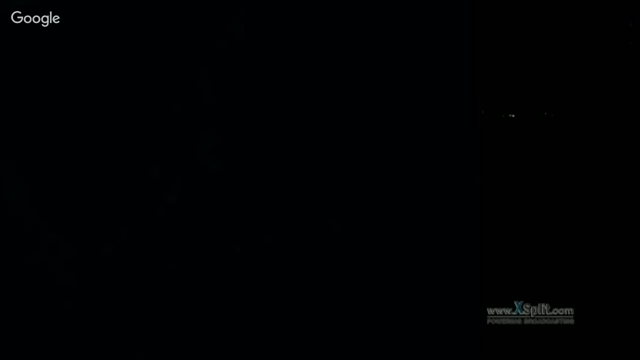 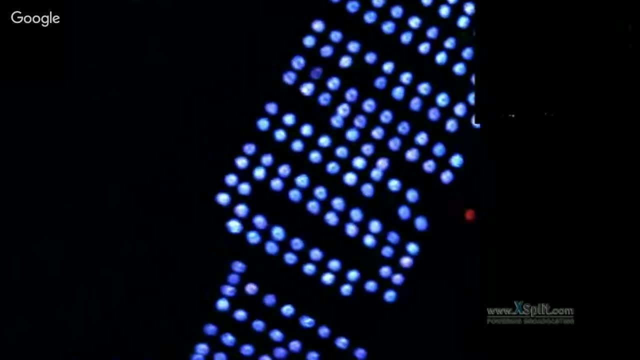 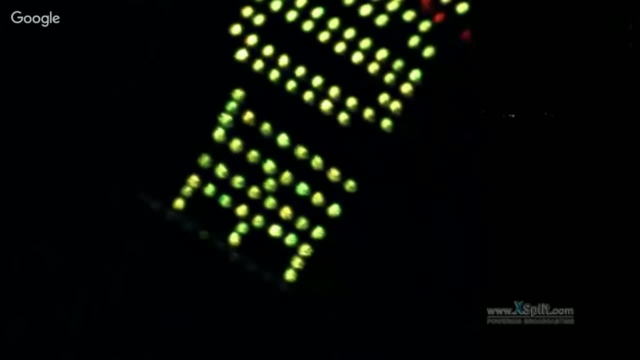 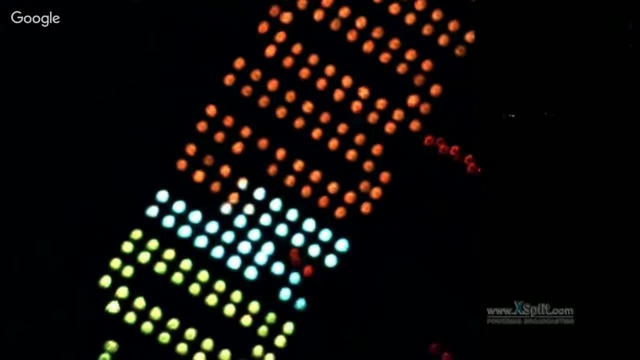 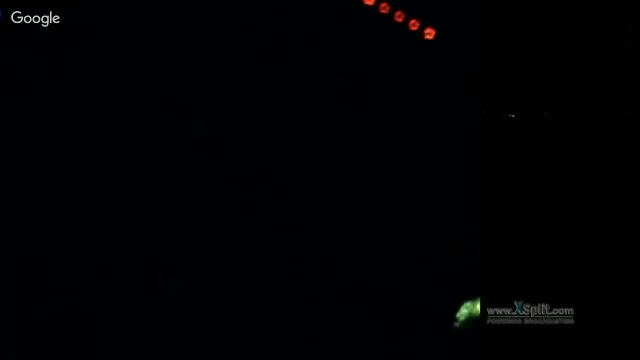 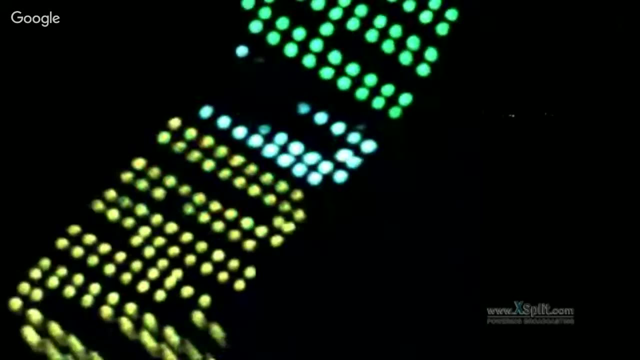 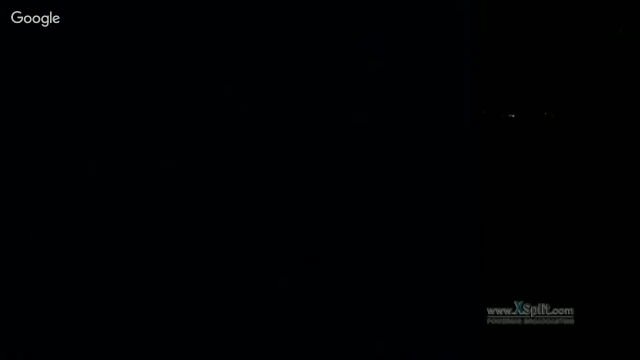 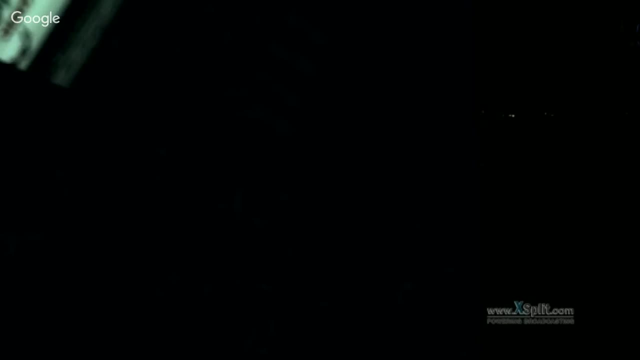 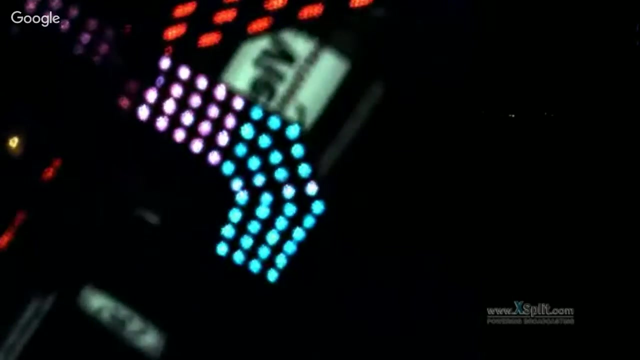 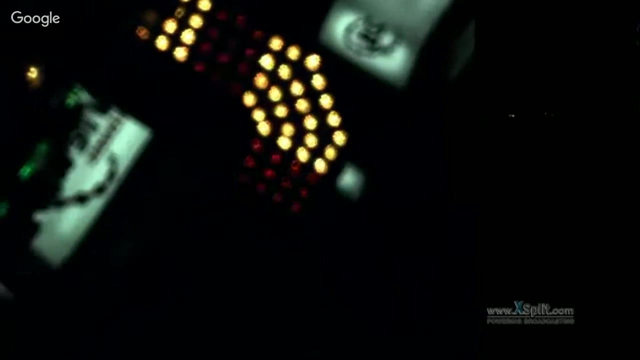 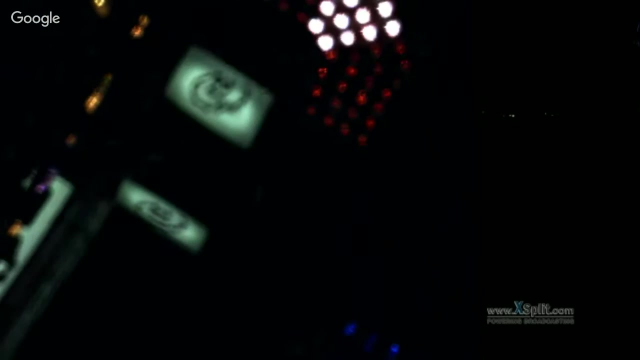 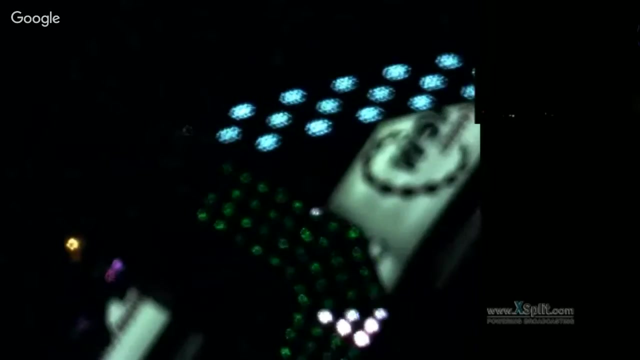 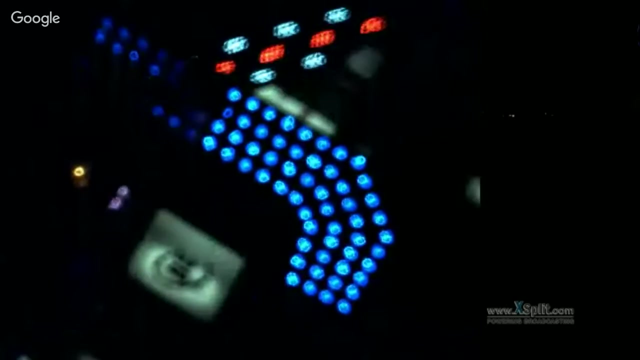 again the something of the moon, again the something of the moon- great stuff, yeah, wow, wow, wow, yeah. yeah, you see my telescope slowly. yeah, you see my telescope slowly. yeah, you see my telescope slowly adjusting. yeah, we can see that mate. yeah, we can see that mate. 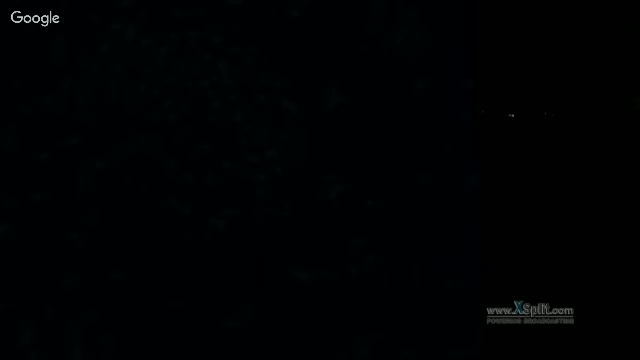 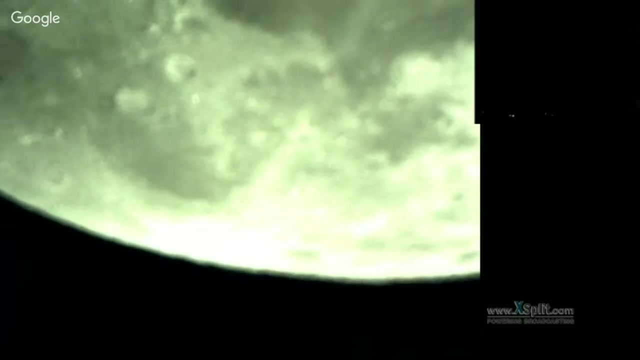 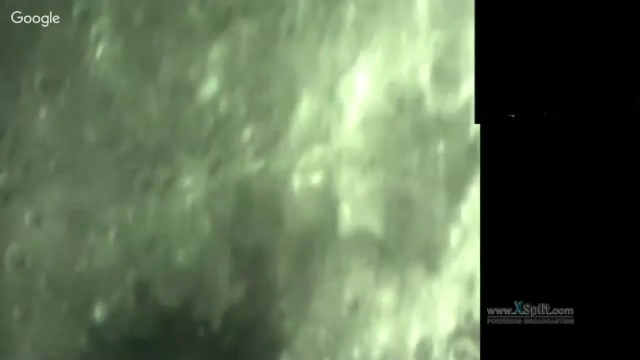 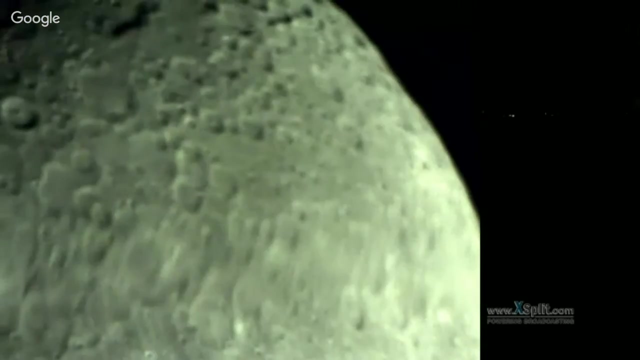 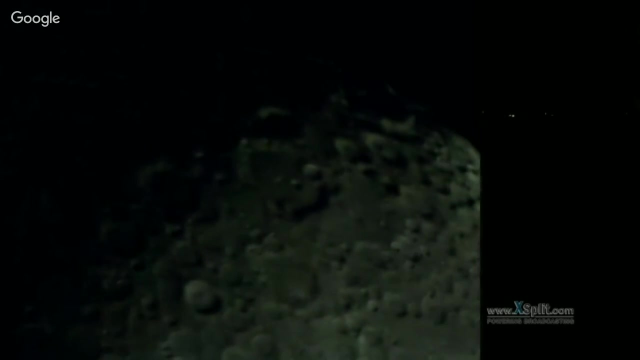 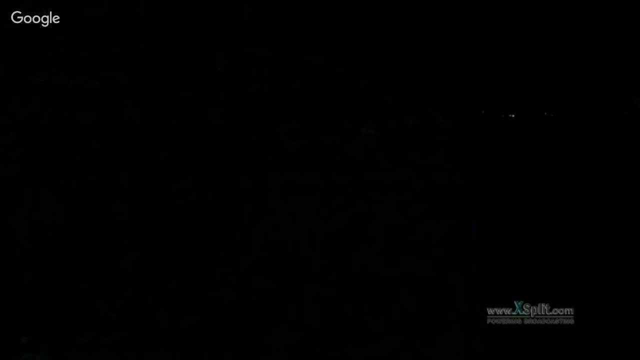 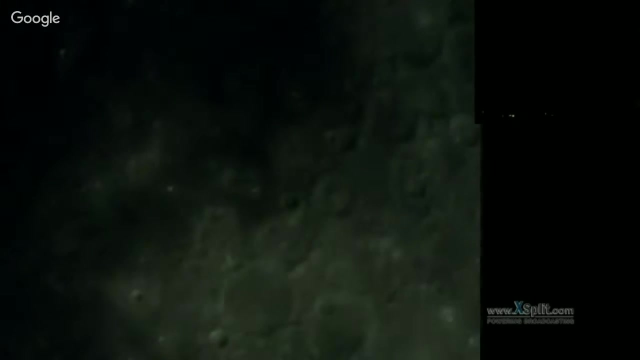 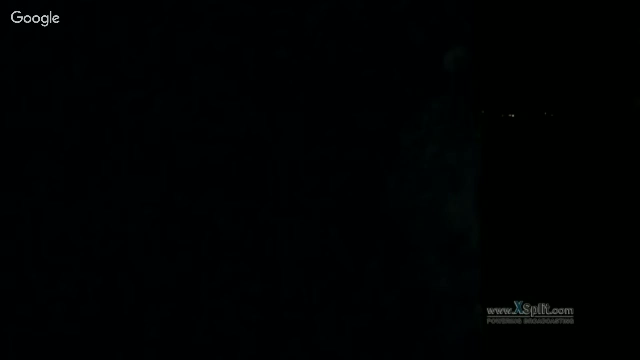 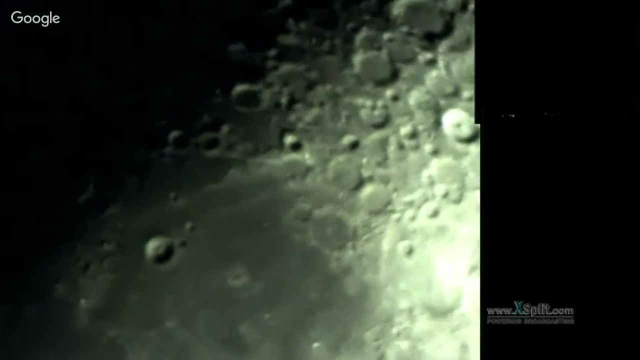 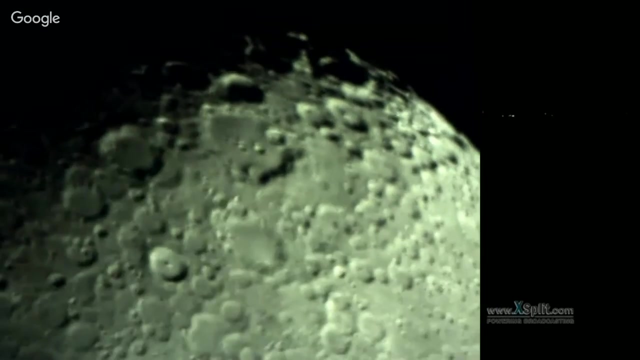 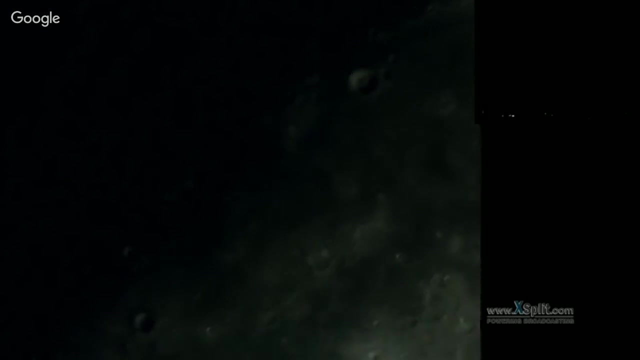 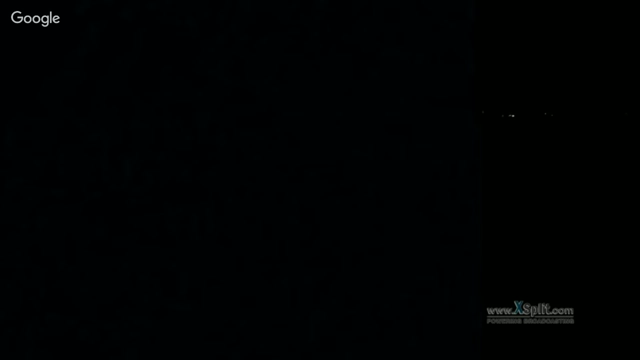 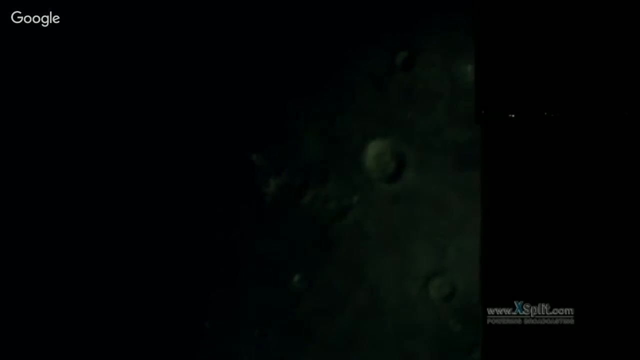 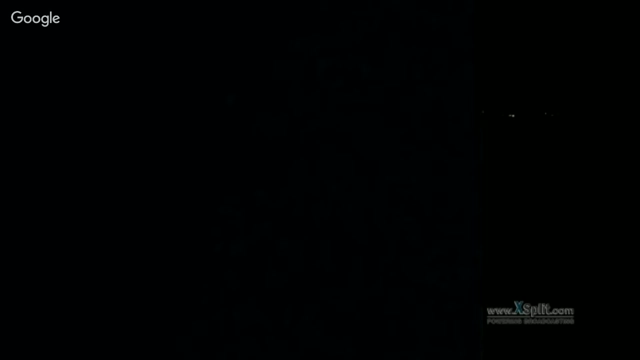 out loud on tonight here There will be, I think, 30 seconds of clear sky in about 10 seconds. So let me try to give you the best. okay, three, two, one. Some really nice detail there, Xander, Yeah, that was it drawing. I was starting to enjoy it. 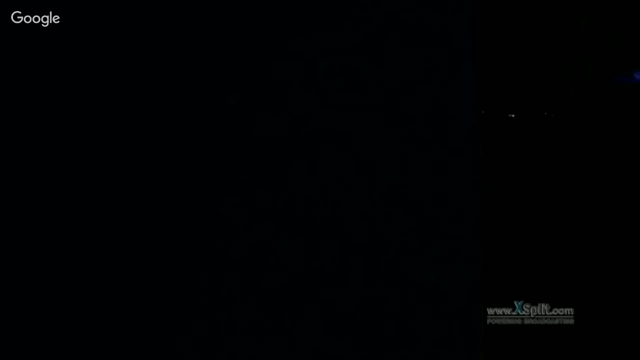 We are getting a little bit better luck than I was earlier on. Xander, Yeah, okay, I will show you some fun stuff again. people hanging in the sky, Okay, Okay, Okay, Okay, Okay, Yeah, you see, like flashes of light, those are people hanging in the sky and cheers. 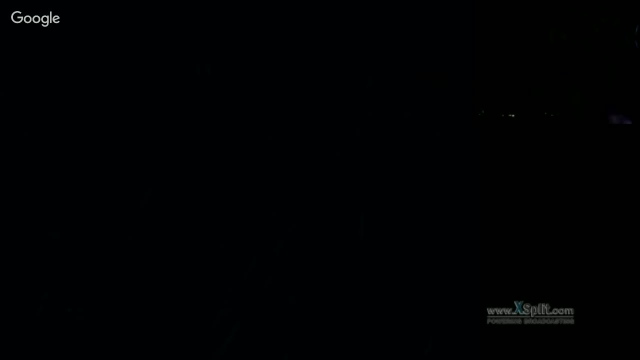 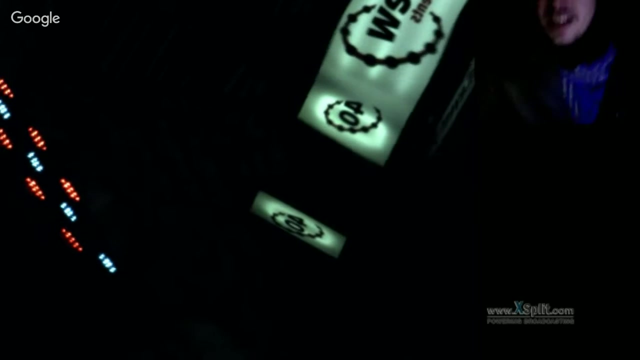 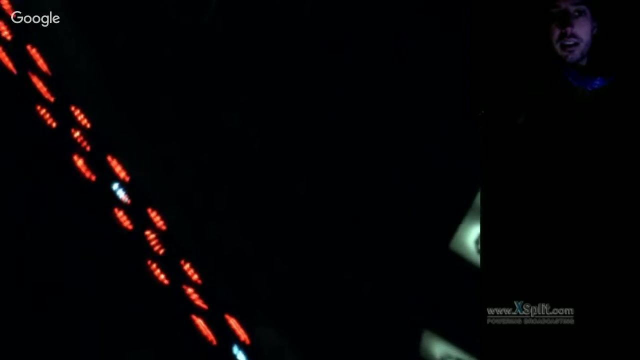 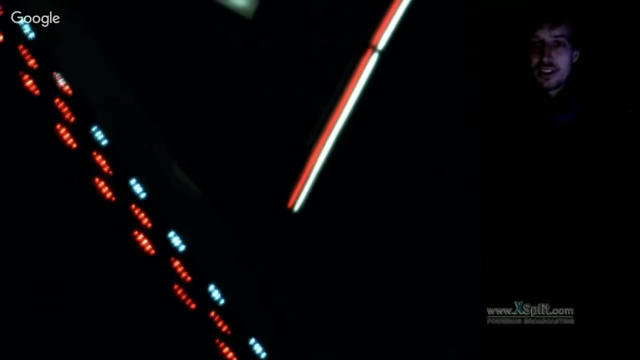 Wow, Really These pink, bluish dots. So there's a ferris wheel and there is a big. now the ferris wheel is was at a standstill. Oh, it's already again turning. I'm showing you the Ferris wheel just because there is no moon at the moment, Hopefully. 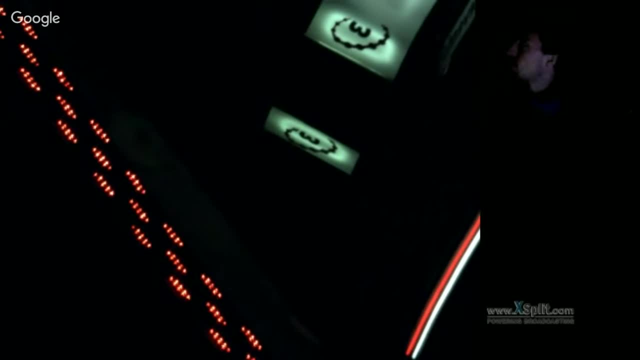 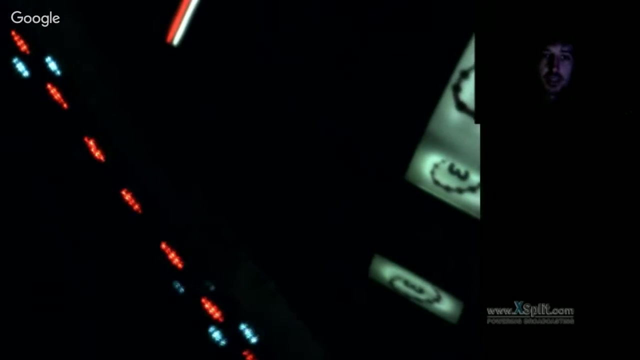 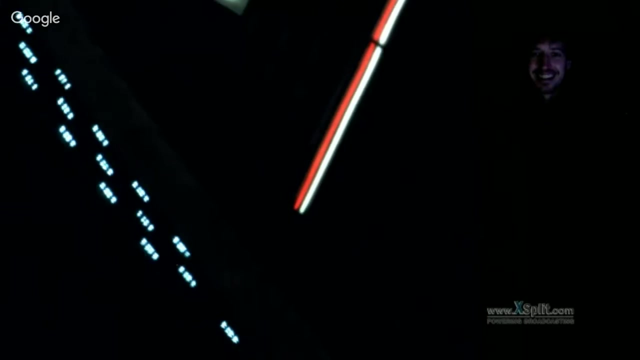 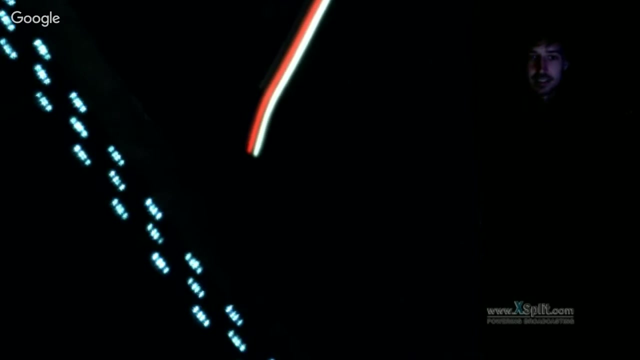 we'll get a clear sky in a couple of seconds. Grant, we will do the talk about the spectroscopy next week. I will be done next week. If not, I'll do it from home. Xander, My internet connection is a different one at home to the observatory. I would prefer to do it at the observatory. 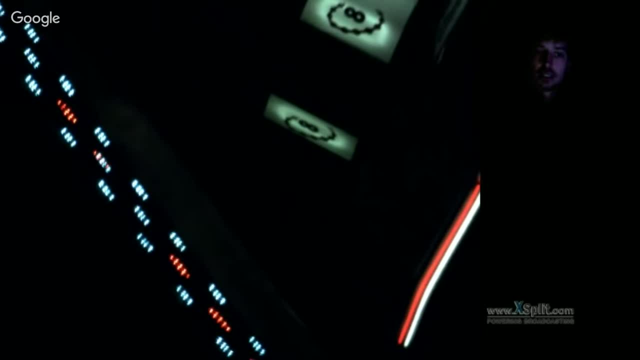 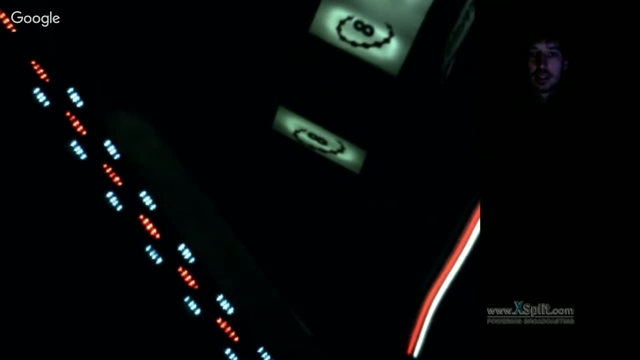 where the telescopes are. I can't bring a portable mount back with me. I can bring one of the Skywatch and EQ6 Pros. We were away doing things last week at the Royal Cornwall Careers and I had all the telescopes and mounts in the car here. What I should have done was just left them here and did. 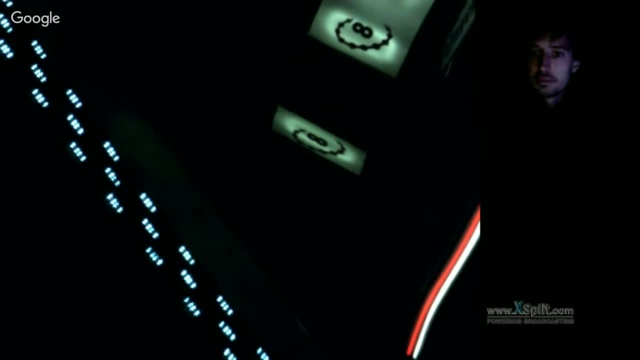 the show from here tonight. We'll see how it goes. Yeah, we'll see how it goes. So, for everyone who is joining this broadcast, you don't see any live moon at the moment. unfortunately, We are having some problems with the weather. 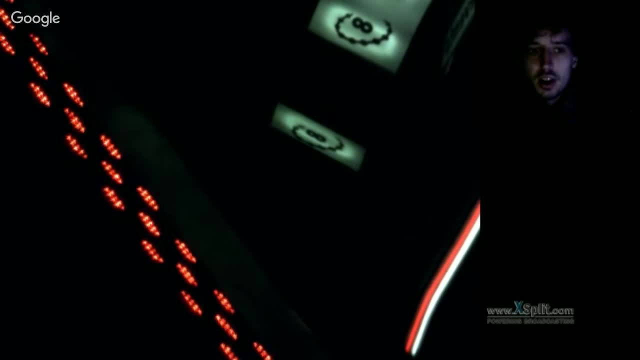 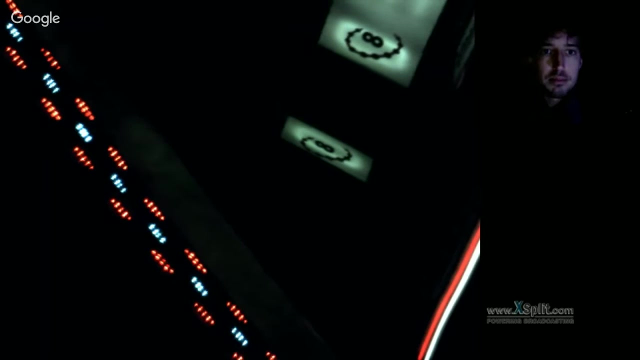 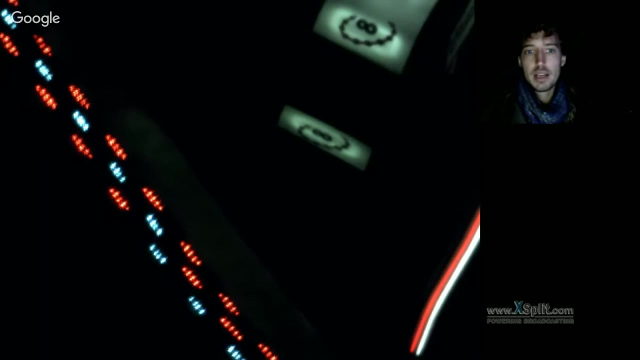 of course, But feel free to ask us a question and hopefully we will be able to answer them, of course, But at the moment the Orionids meteor shower is active, And so you might ask yourself: okay, what can I see during this week? So in three days there is an interesting. 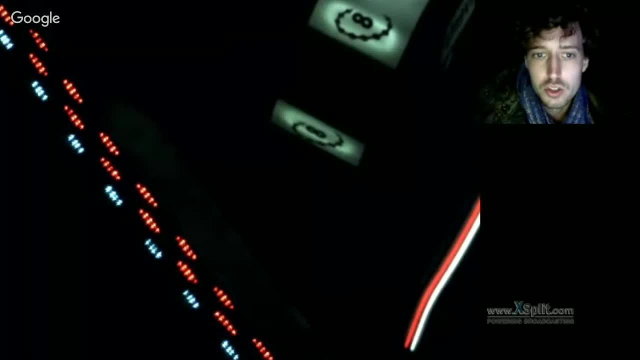 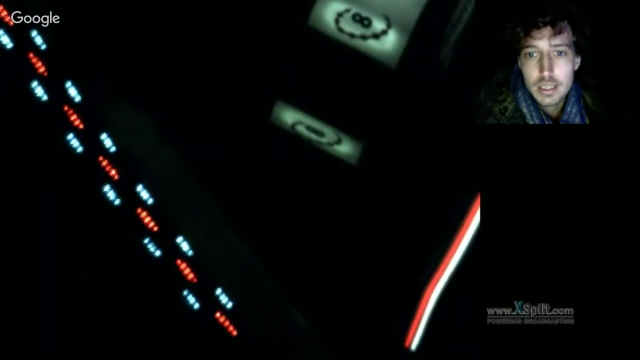 conjunction of Venus and Saturn. Okay, So what can I see during this week? So in three days, there is an interesting conjunction of Venus and Saturn. So, going from Pluto to Venus and the planet Jupiter, those two bright planets will only be one degree up, although not as close as the conjunction on the first of July in this year. 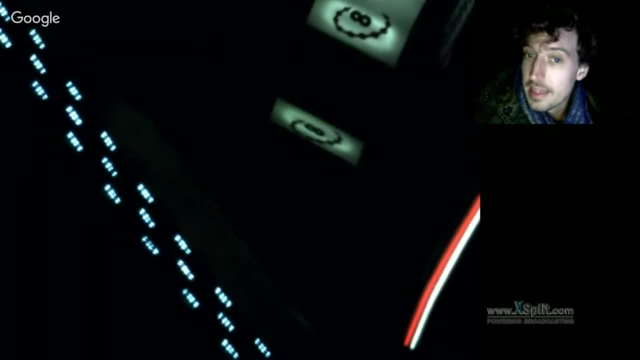 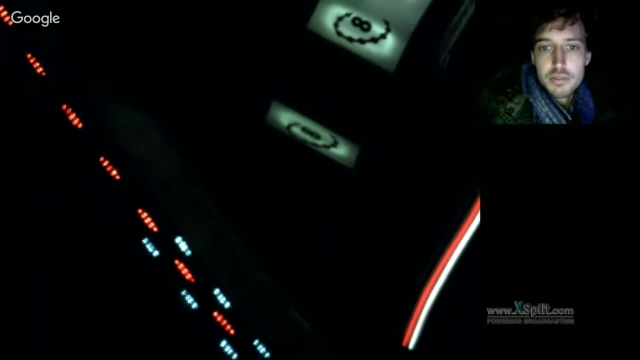 That conjunction was really close because these two planets were in 3 degrees of proximity to see and it's quite relatively easy to take pictures of it Without a telescope. with a DSLR camera you should be able to make very beautiful pictures of conjunctions and that's a really interesting start as a beginner. 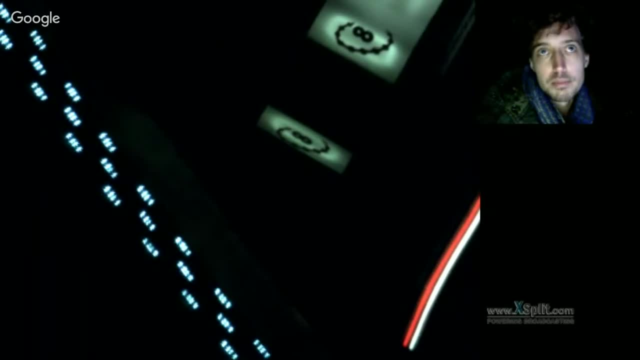 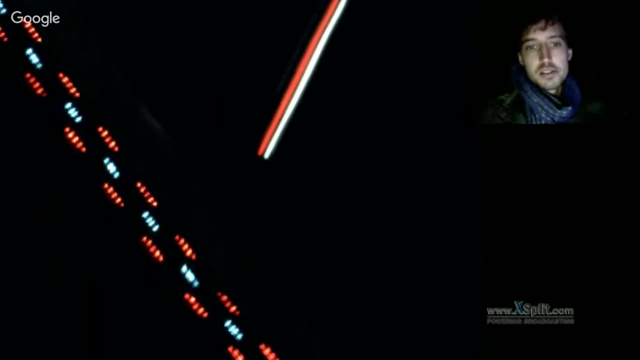 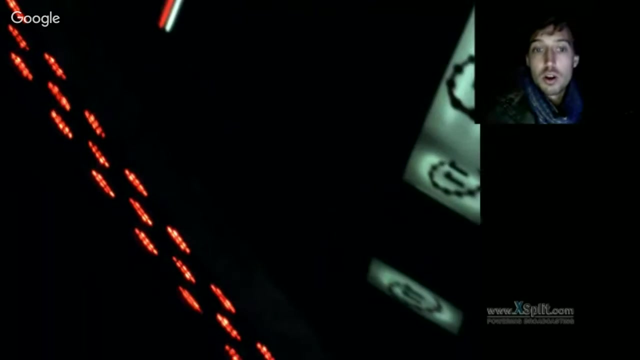 in astronomy. What is conjunction? Well, that is when two planets are in the night sky, close, in close proximity of each other, in when you see it, and you speak of the conjunction, when it is five degrees or less distance, visible distance. so that's on October 25th. one day later, on October 27- sorry, 26, there is an 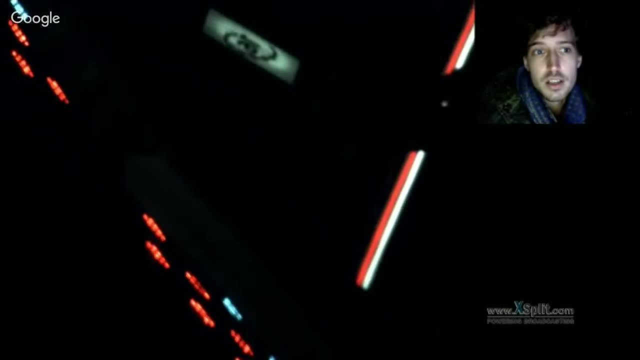 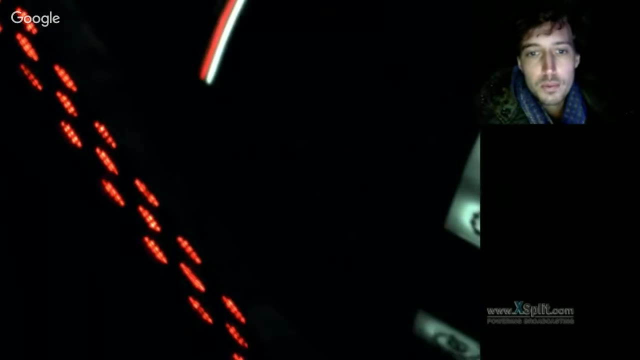 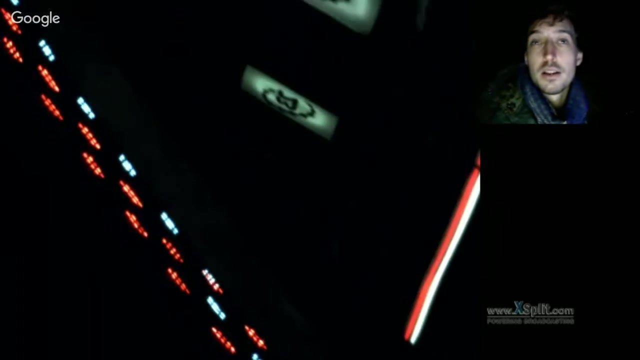 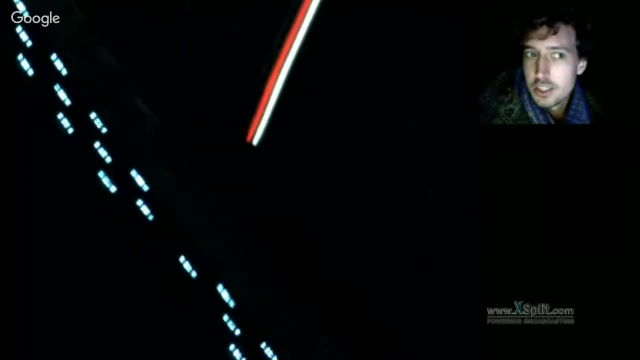 occultation of the planet Uranus, or Uranus- sorry, Uranus- by the moon, and it's visible for observers in New Zealand. so you, Uranus is a quite well it's. it's a difficult planet to spot but it is very interesting because you see some greenish tint and the moon. 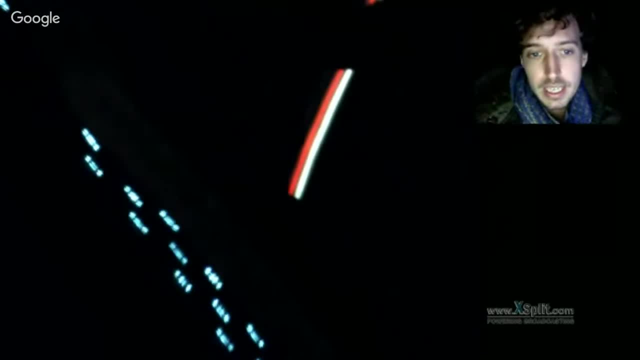 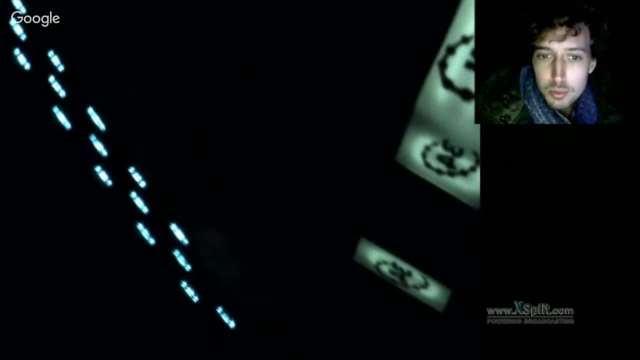 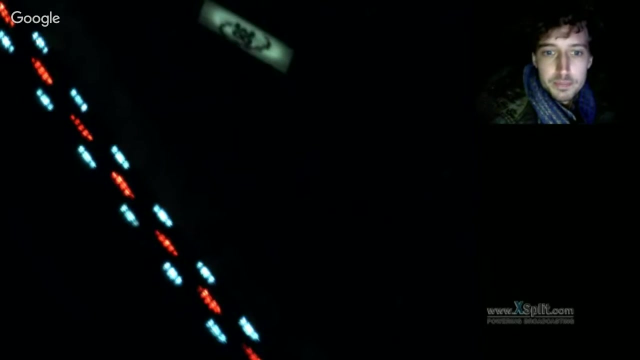 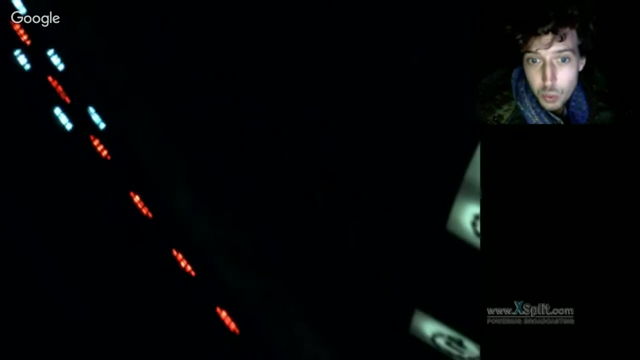 will block it when you're living in New Zealand, so we hope people from New Zealand are able to broadcast it from there. On October 27 there is another supermoon and, if you were watching these broadcasts, earlier on as well, we did a broadcast by the supermoon. 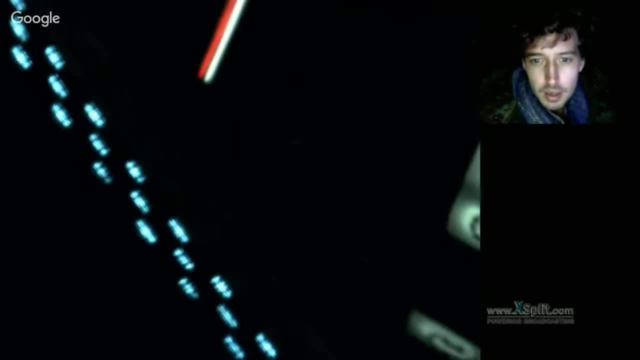 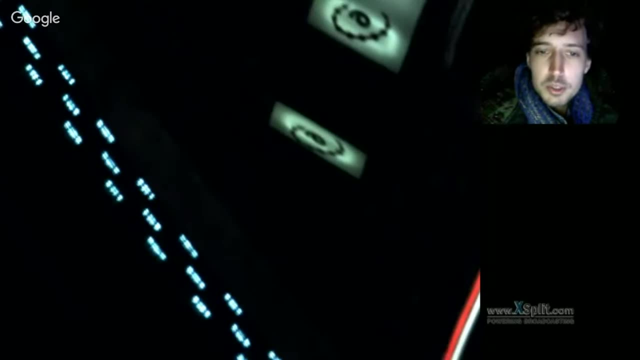 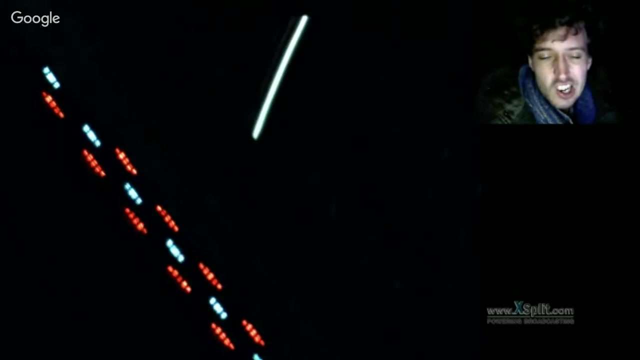 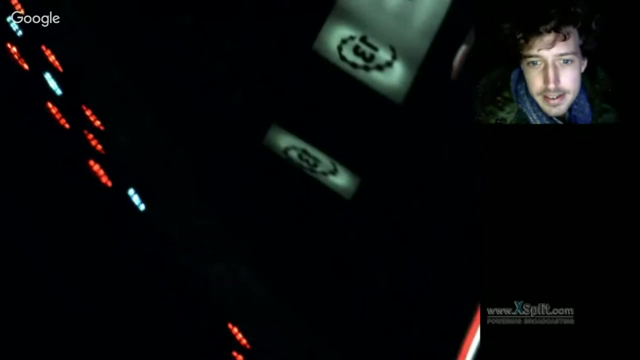 but what is actually supermoon? well, that is the平安, because when the? well, let me try to to give you a different approach, because in 2015, there are three super moons, and we already got number one and number two. and when does a supermost happen? well, that, happens when the moon is really close and it is the one who lives inód happens when it is closer than 261.800 kilometers close to our earth. the largest super moon of 2015 happened on september 27, and then the moon was 356 000. kilometers close, and now it is on october 27th, it is 359 000 kilometers close, so it's about 2500 kilometers farther away than the first or the second- sorry, the second- super moon, which you should be very accurate when you notice the difference. so a super moon happens when: 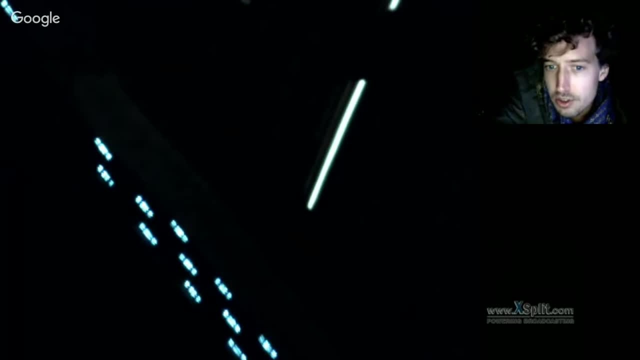 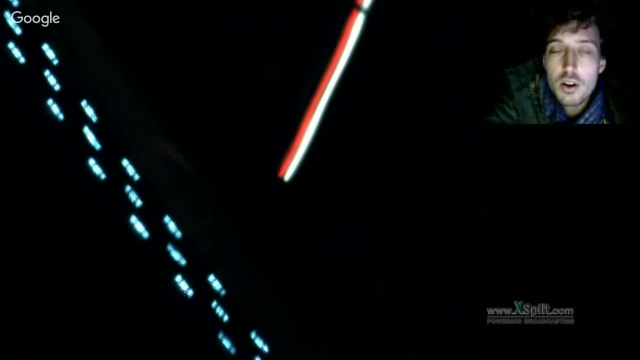 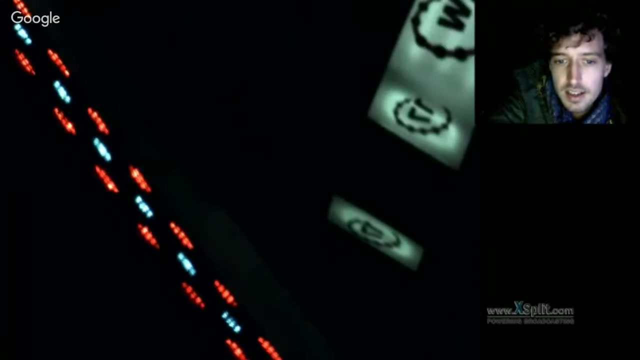 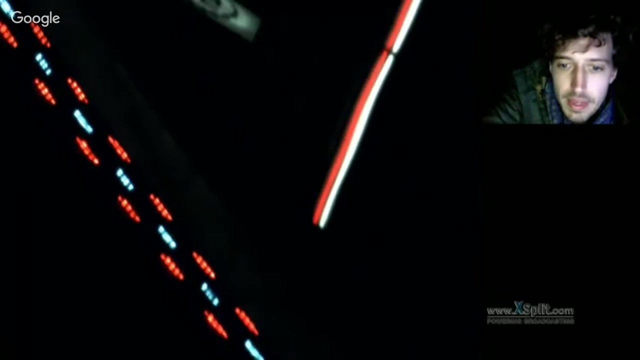 it is close to earth because it doesn't make like a sir, a perfect circle around the sun, but it are around the moon, but it's more like an ellipse, um, and that phenomenon coincides with a full or a new moon, and when it's closer to specific 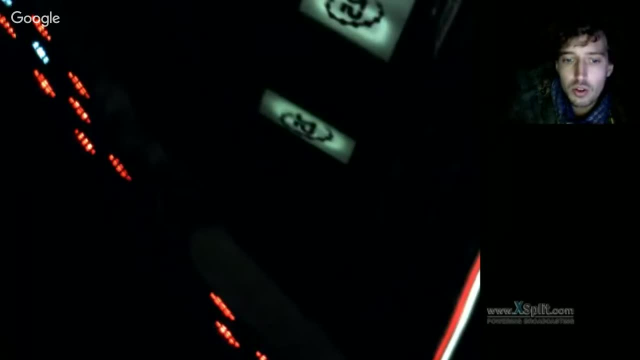 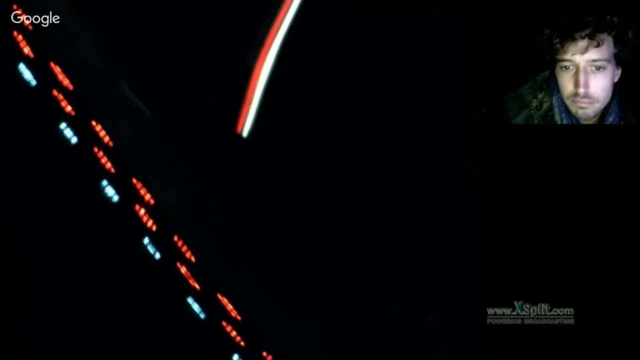 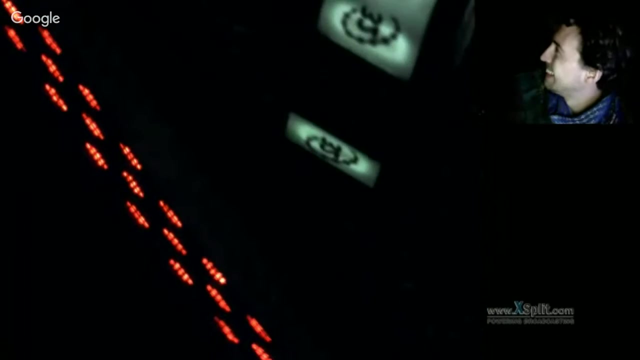 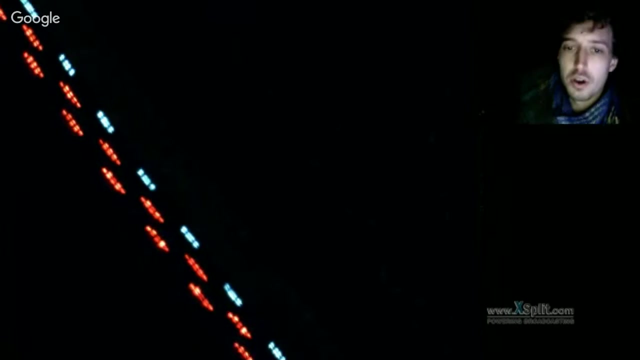 distance what i already told you. it is called a super moon, so that happens on october 27th, um, so i'm, of course, when the weather permits, i'm definitely trying to show that to you. when i look at my right, i see here some uh parts clear sky, so hopefully i will be able to show you. 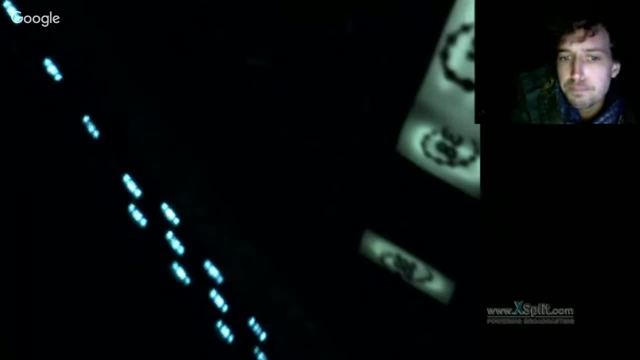 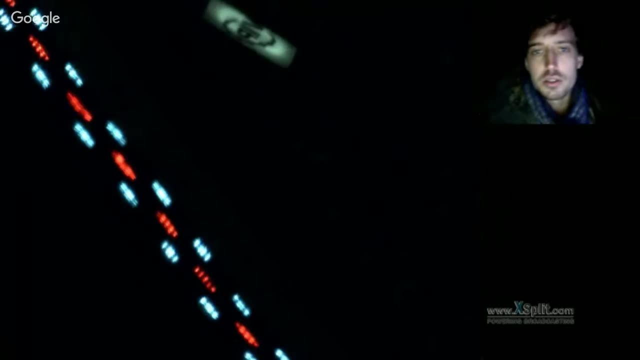 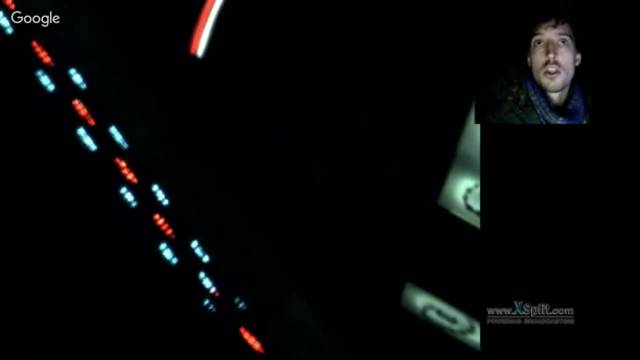 the moon in about 10 minutes or so. um, i'm going to show you the moon in about 10 minutes or so. um. going back to what will be visible upcoming week, in six days, there will be an interesting conjunction of planets: jupiter, mars and venus, so triple conjunction, those three. three planets are: 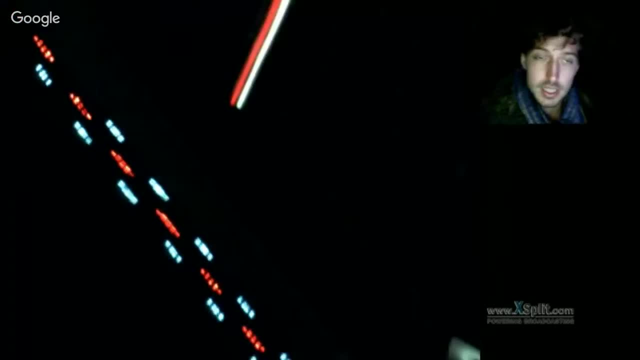 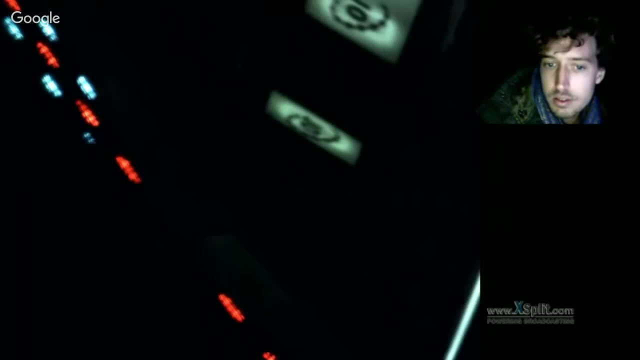 within five degrees of each other. so that's very interesting, and you should try to catch it on camera. it's very easy, you don't need a telescope for it. you did, you. you should be able to make some beautiful pictures as you go along. um, so that's it. um, if you enjoyed it, please leave a comment. um, if. 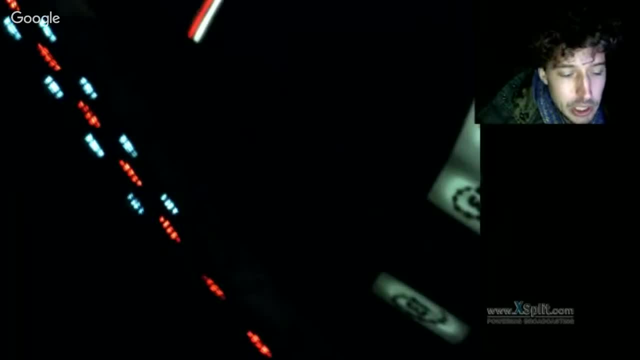 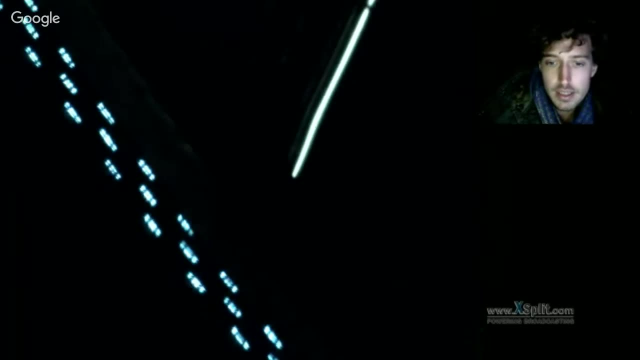 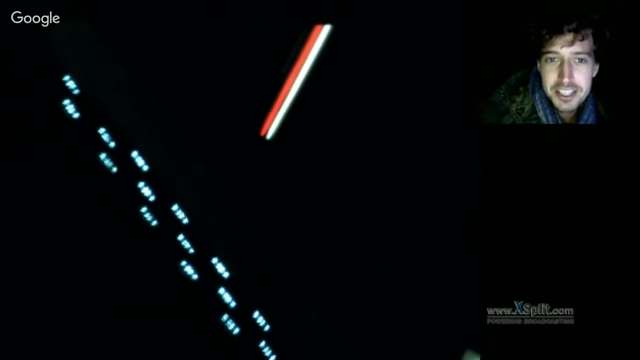 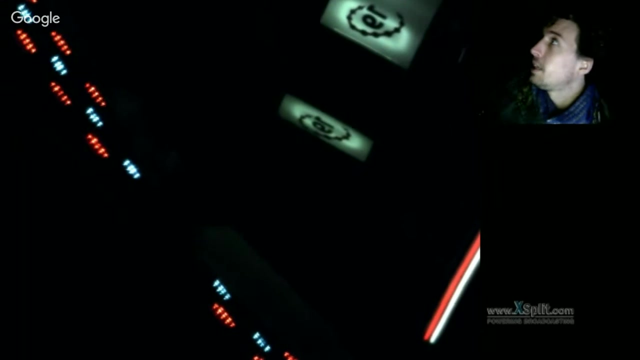 using a DSLR camera and very interesting. one of our broadcasters, Benjamin Eunice, is a young broadcaster from the United States and he was planning to show the supermoon, or sorry, the Jupiter, Venus and Mars conjunction live on Astronomy Live as well. Hopefully he will be able to do that and weather is. 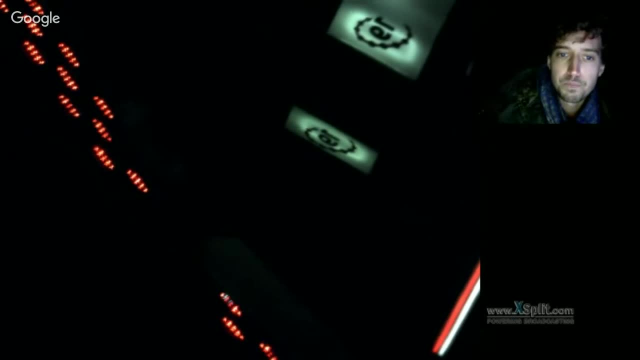 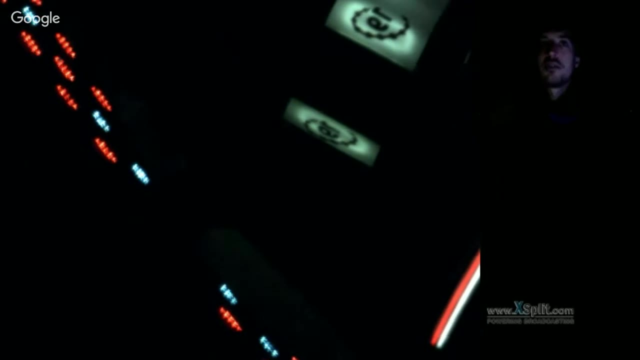 playing ball at his location. Yes, so that's what's upcoming, and you see that the ferris wheel- it is just stopped again. There is a carnival here in Amsterdam and you hear the church, with a lot going on. So, Grant, I have a clear patch of sky. It's not very bright, but I think we should be able to get a few minutes of light. 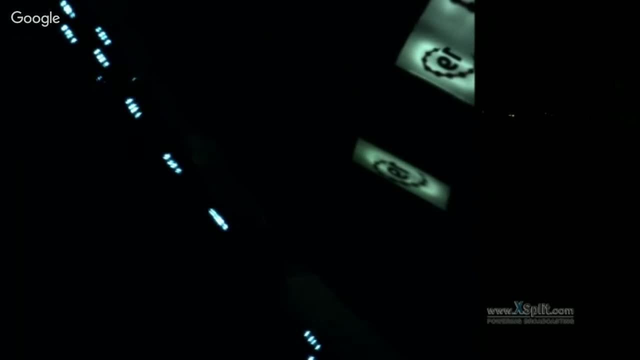 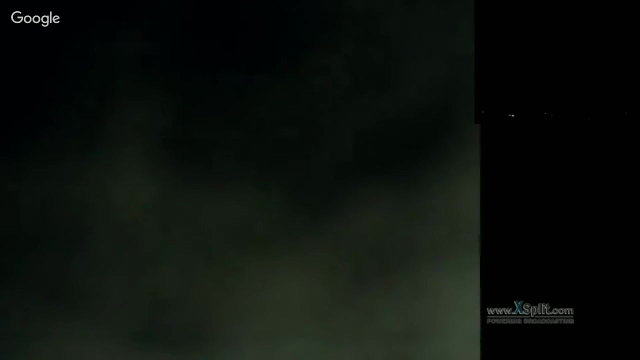 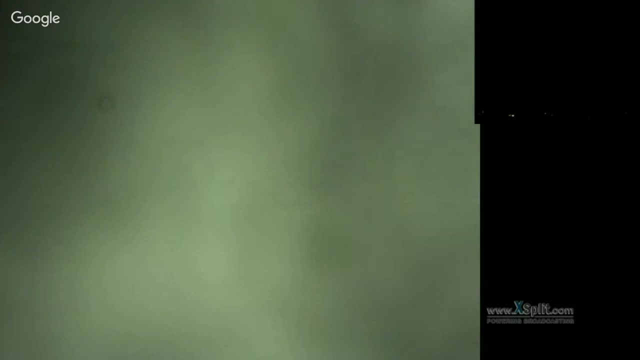 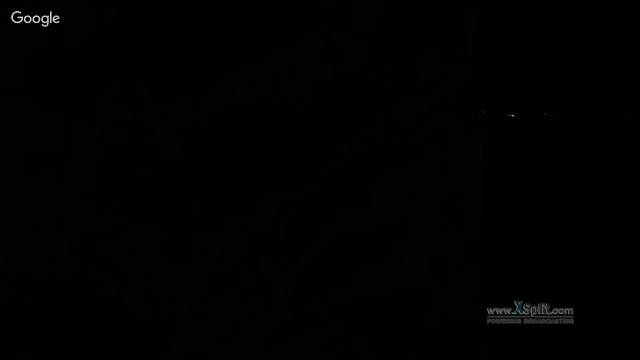 Well, it's a lot clearer than I've got weather here, wise Xander, so any moon's good tonight. I'm going to go ahead and turn it on. Let's see if we can get a T minus 10.. About 20 seconds of clouds left. 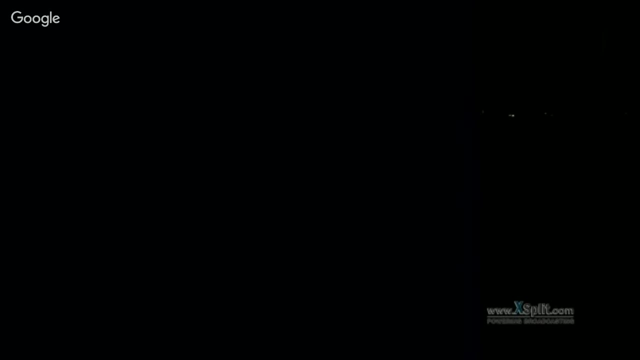 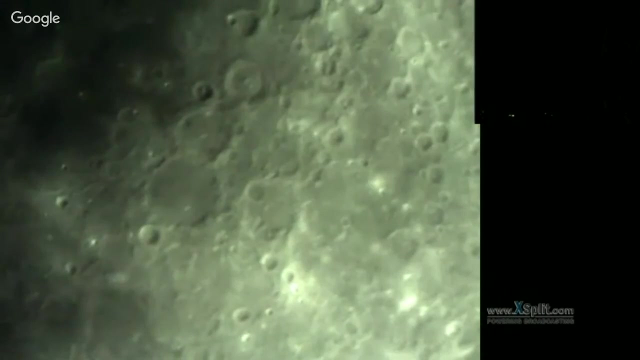 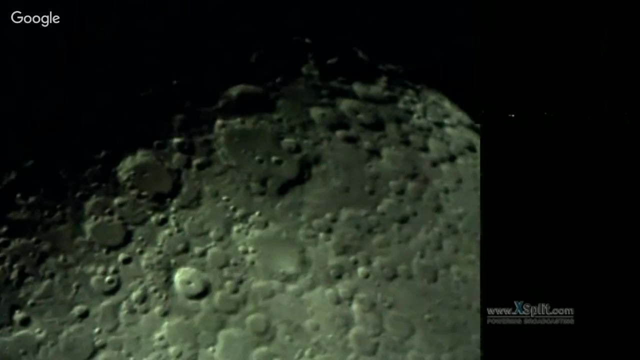 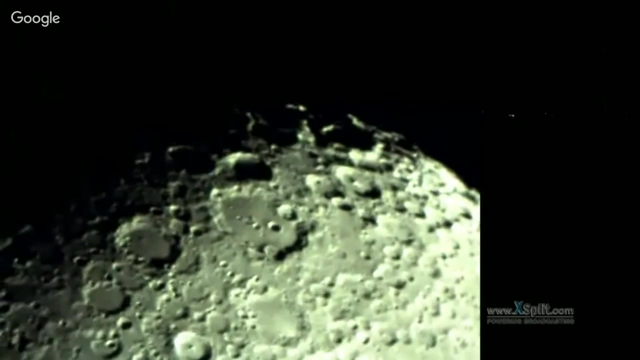 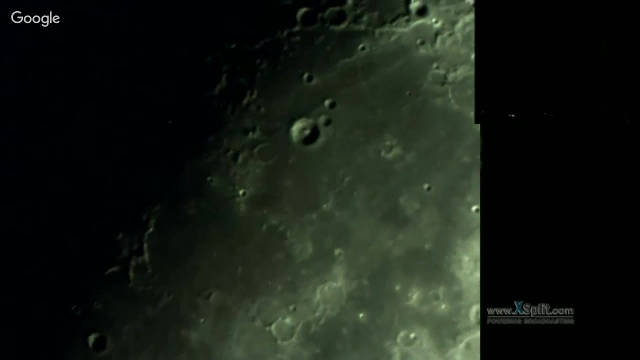 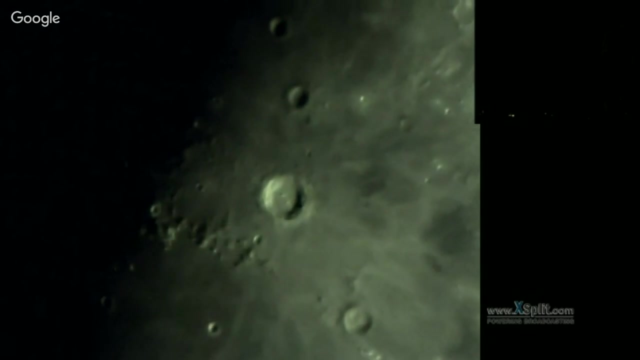 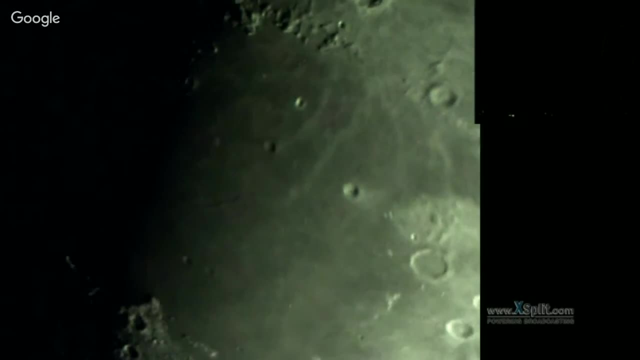 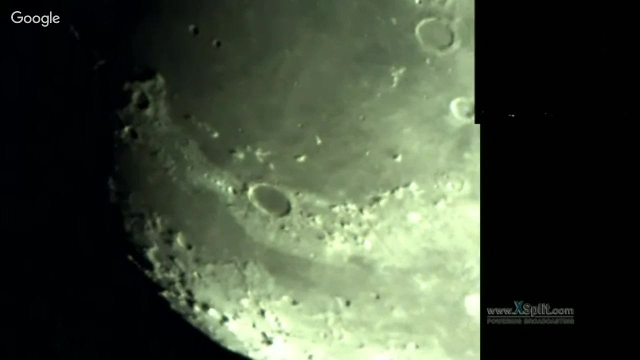 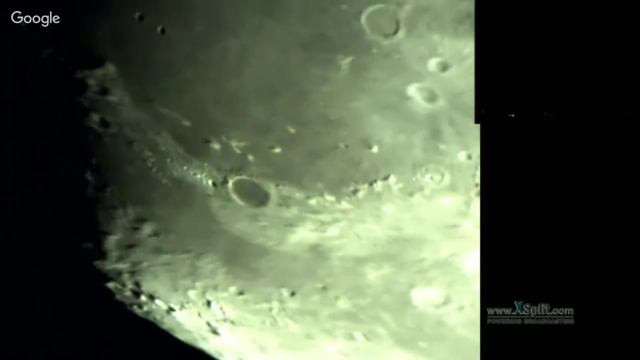 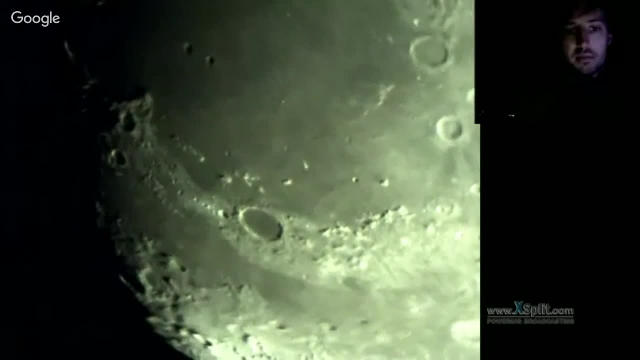 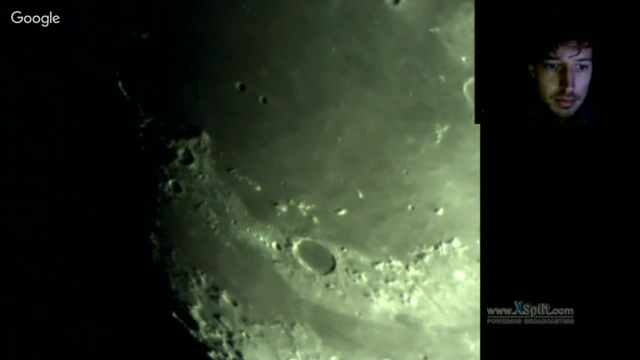 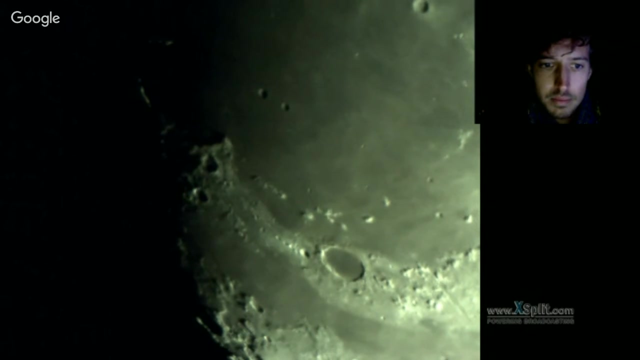 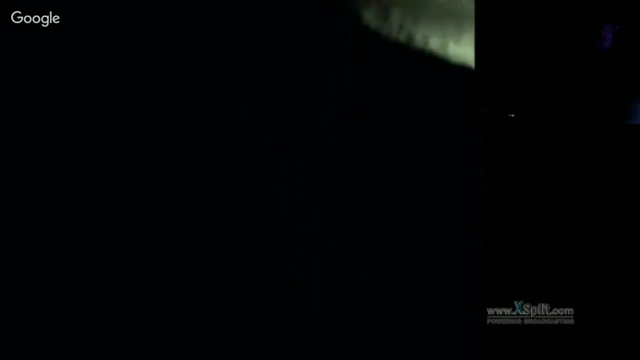 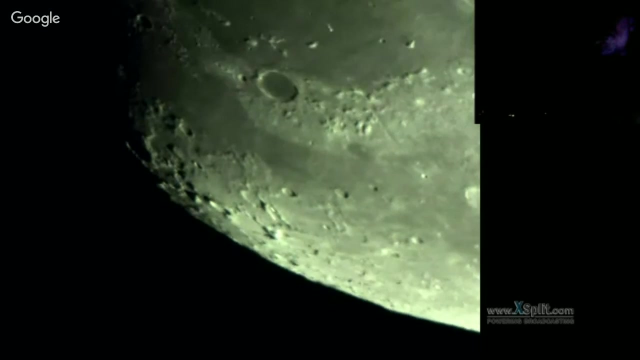 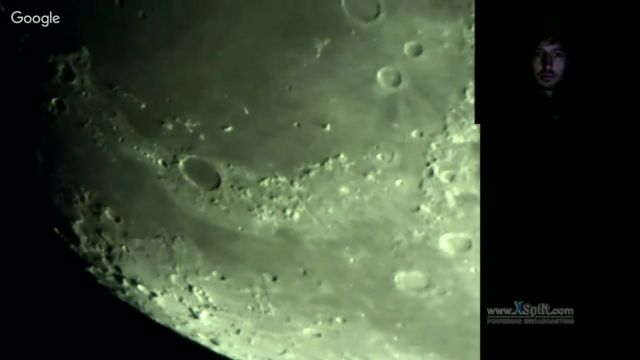 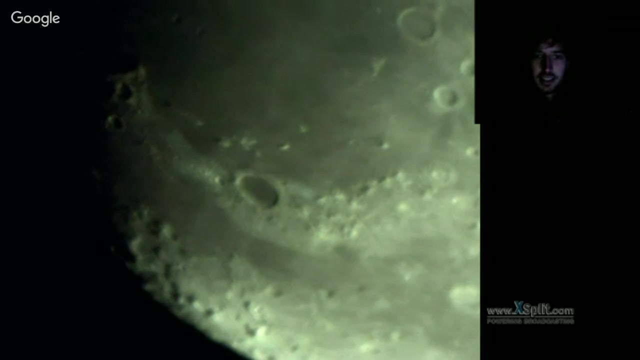 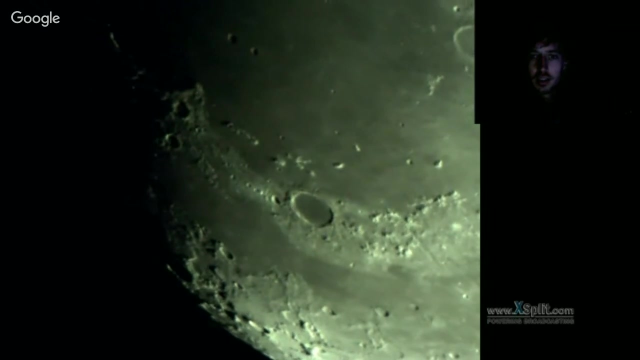 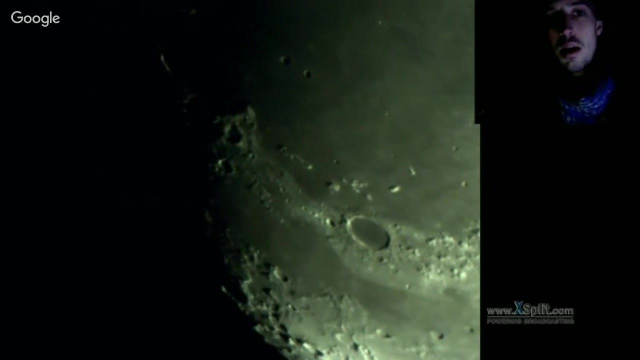 That looks fabulous. Wow, yeah, that looks really good, zondo. yeah, oh, look at it. nice detail there. yeah, man, look at the beautiful ghetto in plato. yep, that's what i'm talking about. wow, you see the, you see the, the top of the hills in scary uh, sorcery even. yep, you can see that. 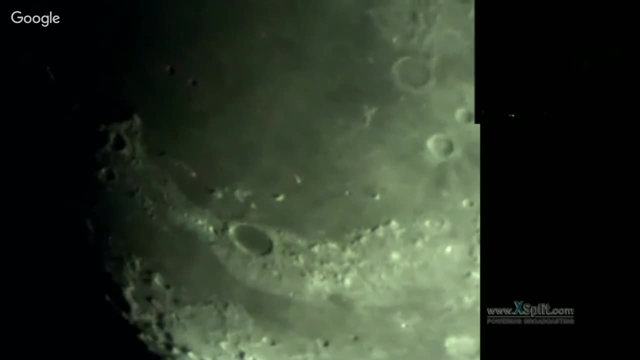 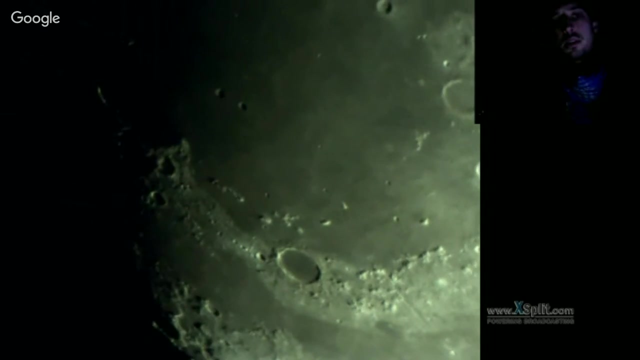 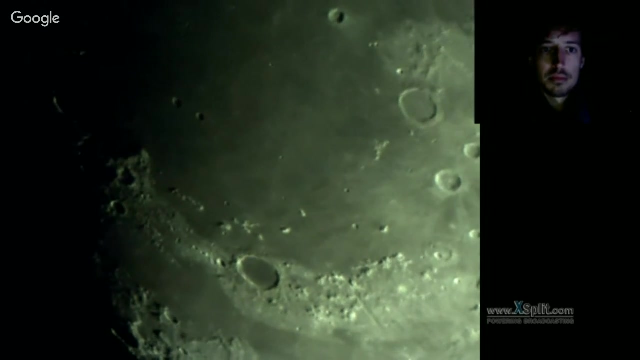 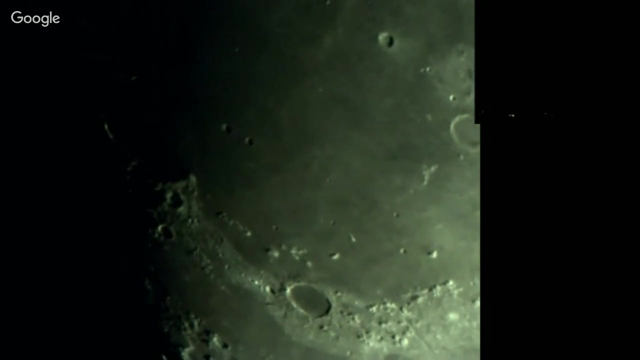 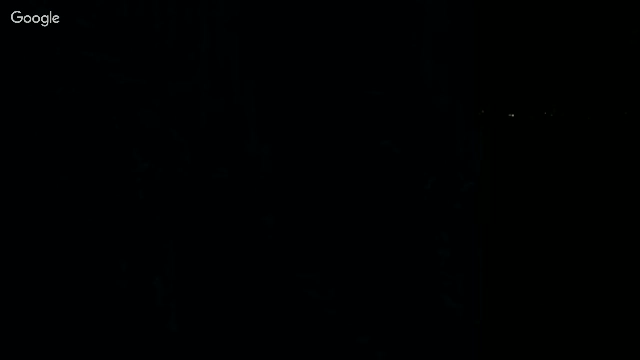 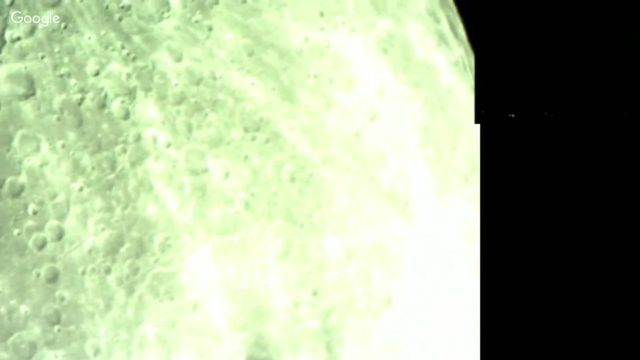 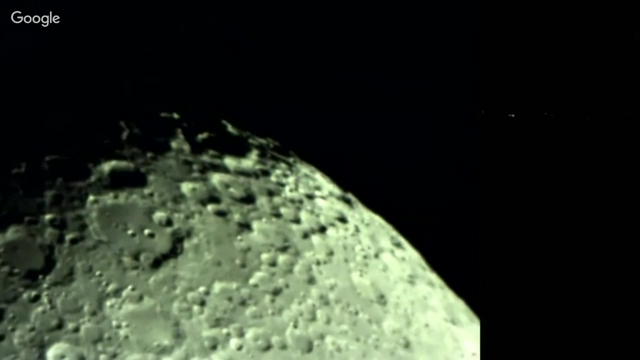 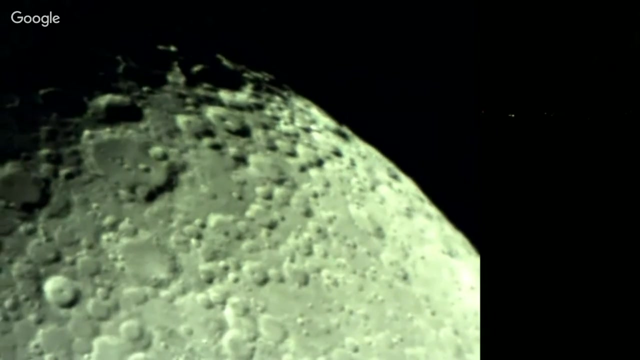 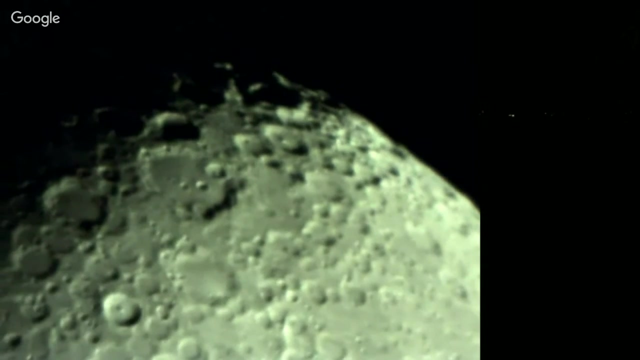 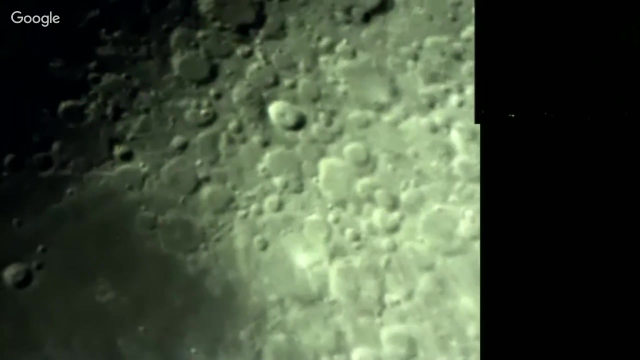 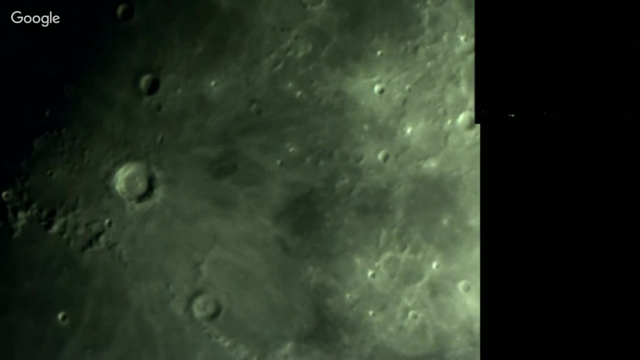 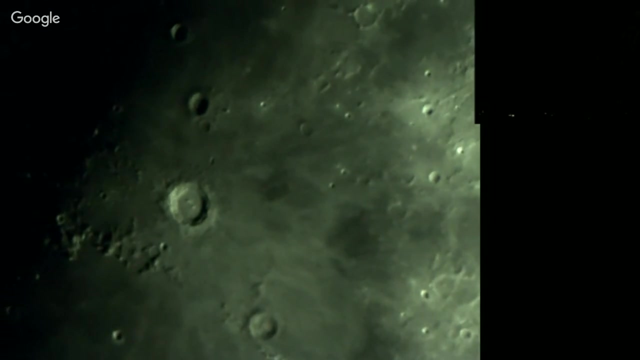 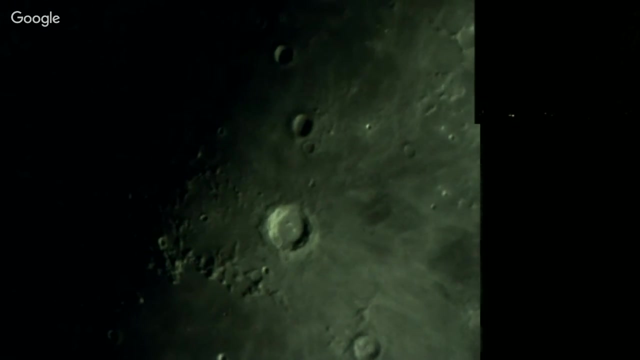 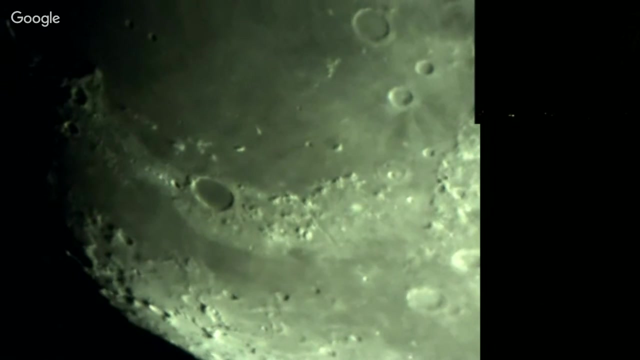 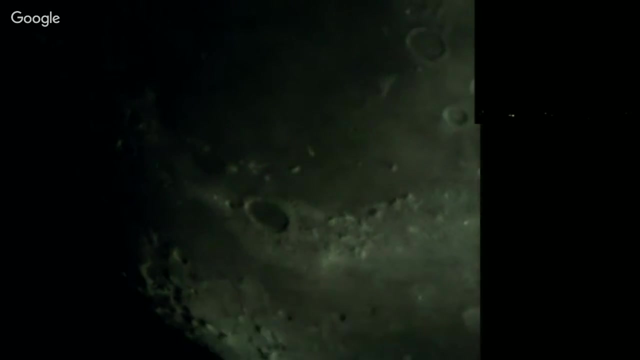 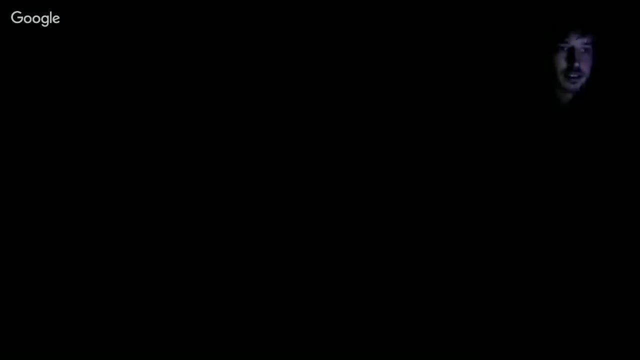 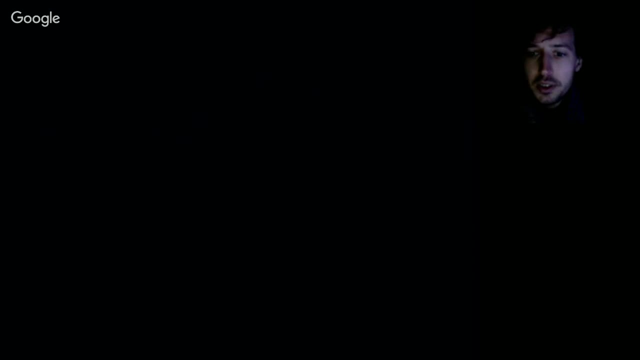 And we will be happy to answer them. If you are an astronomer and you're watching this broadcast, feel free to join our show during this one Or one of the shows next week. We will be live every Thursday on 8 o'clock Universal Time. 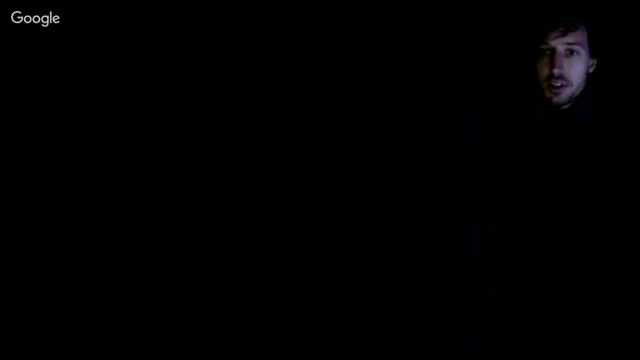 And we will talk about a different subject. For example, next week we are Well Grant McIntosh, the other astronomer in this show who just left, will be able- Will talk about spectroscopy And that's measuring a star. 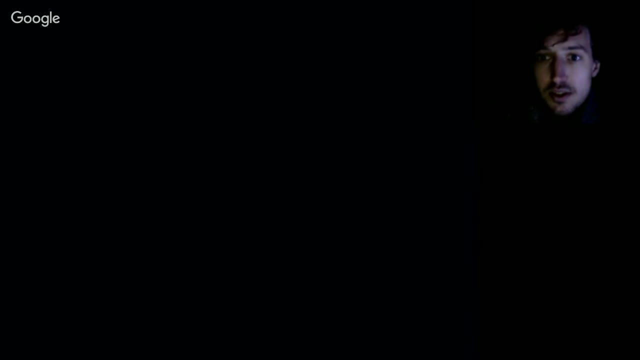 And measuring All the substances that are part of that star, And you can also measure the temperature. He will tell about the basics of spectroscopy, Which is part of physics in astronomy, So actually astrophysics, And Well, I'm looking forward to that. 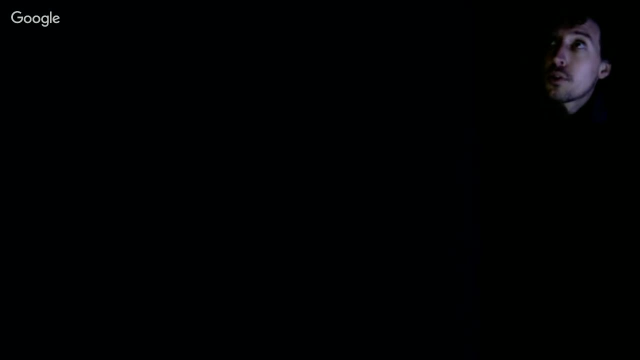 Unfortunately, he's not able to talk about that this week And we will talk about that next week. So every week we will be talking about a different subject And you're happy. You're welcome to join this show And ask questions or join. 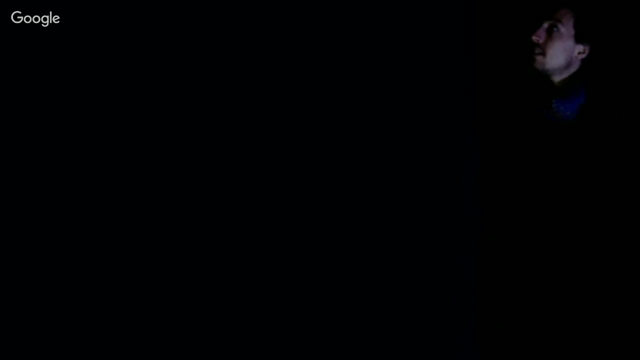 Or just watch. of course, We're dependent on the weather, So that's a thing we can't control, unfortunately, But we are creating an international platform of telescopes. Astronomy Live, And this international community of professional and amateur astronomers should be able to show you and tell you a lot of interesting stuff. 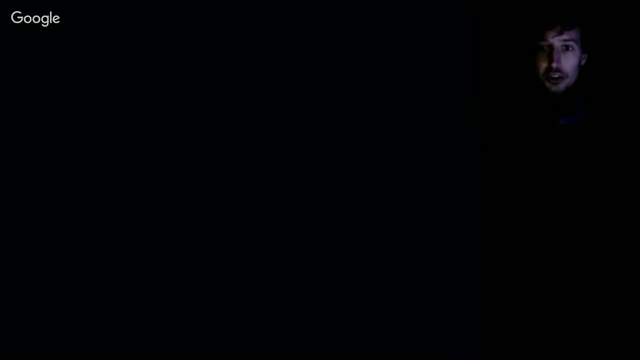 about the night sky, Like we are doing here. So that's Astronomy Live. That's Astronomy Live And hopefully you enjoy this service. It's free And it's You're welcome to join. Don't forget to share this with your friends, of course.